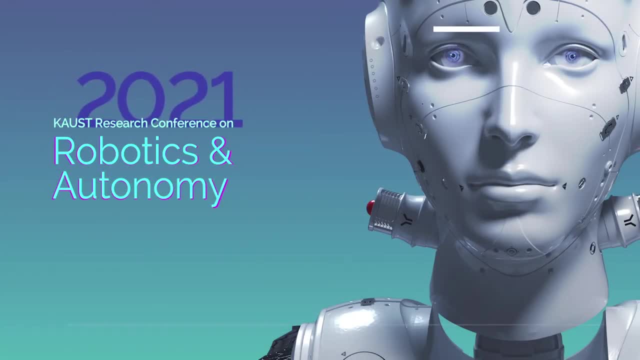 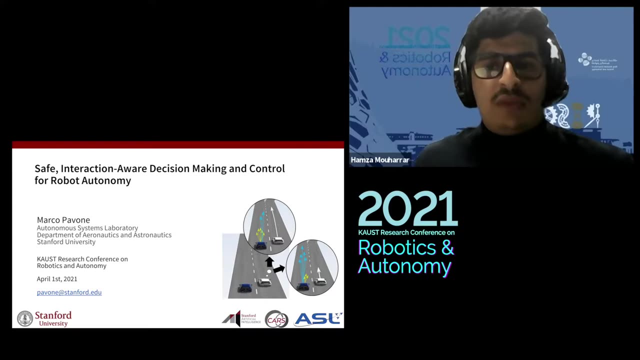 So our next speaker is the Professor Marco Pavone, who is an associate professor of aeronautics and astronautics here at Stanford University. So Professor Pavone will present the decision-making and control stack for human-robot interactions by using autonomous 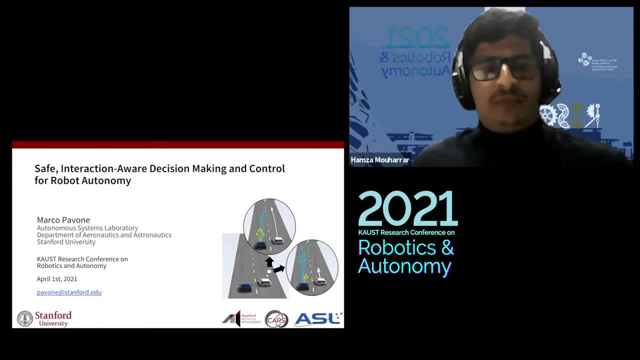 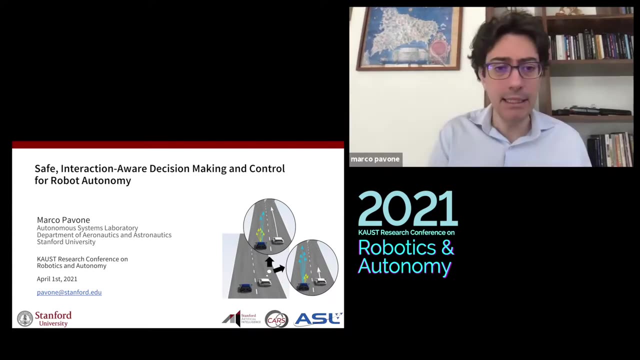 driving Professor, the stage is yours. Thank you very much for the kind introduction. It is a pleasure to be part of this conference. My name is Marco Pavone. I'm a faculty at Stanford in the department of aeronautics and astronautics, where I lead the autonomous systems lab- My lab. 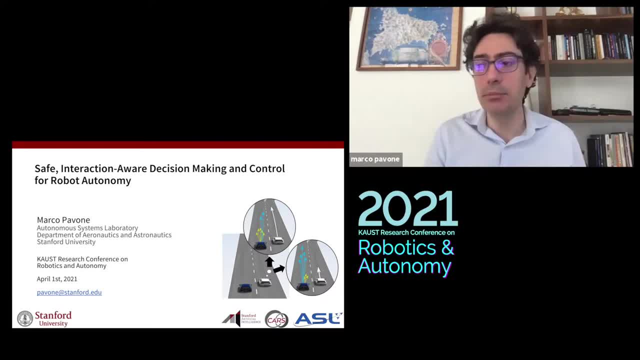 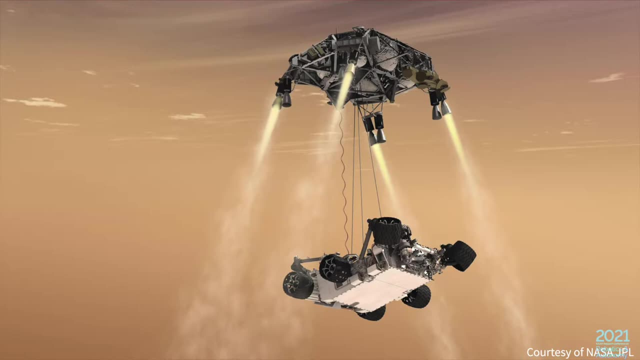 broadly focuses on the design of planning decision-making algorithms for autonomous robots By leveraging and blending techniques from optimal control and machine learning. A key application domain on my work is space robotics, Specifically as a research technologist at the NASA Jet Propulsion Lab before joining 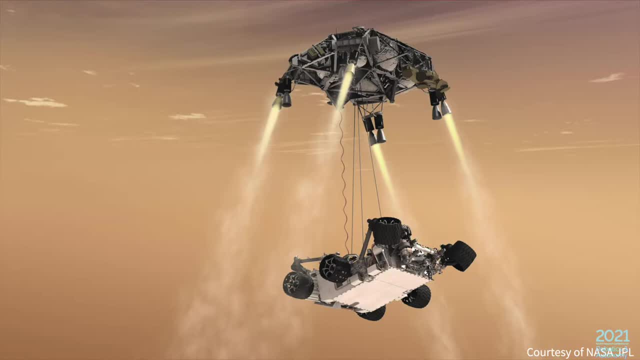 Stanford back in 2012,. I worked on optimizing the entry, descent and landing of rovers on the Mars surface. So for me, a few weeks ago, when the Mars rover successfully landed on Mars, was a moment of relief, since it worked. 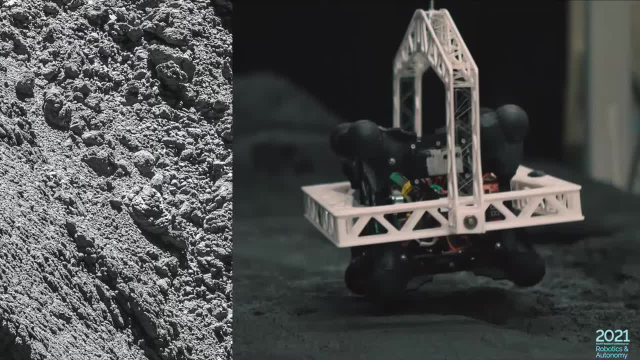 Beautifully. I've also been working on the design of robotic mobility platforms for the exploration of very low-gravity bodies such as asteroids and comets, Where traditional mobility systems based on wheels do not work well due to the very low-gravity environment. 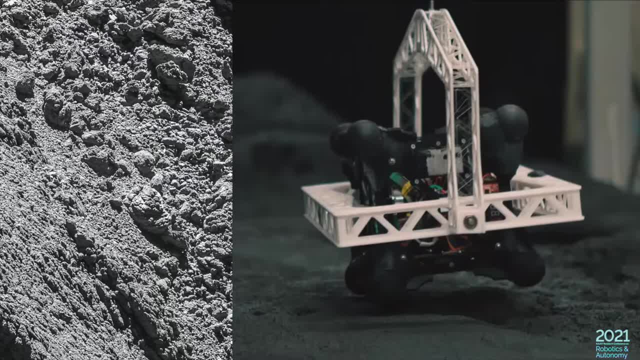 and the complex topography of the environment makes mobility very challenging, Such as in this picture on the left, where I'm showing the typical surface of a comet. In particular, in collaboration with JPL, we have designed internally-actuated mobility platforms which we tested on a microgravity testbed. 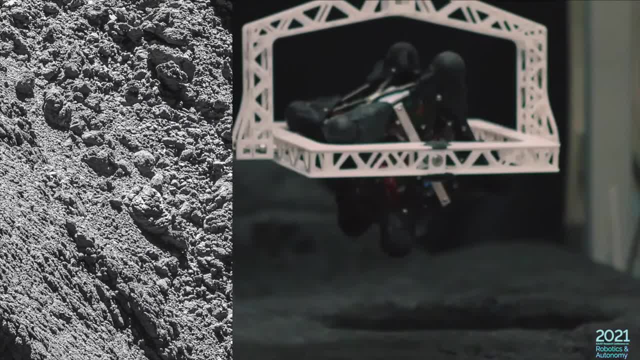 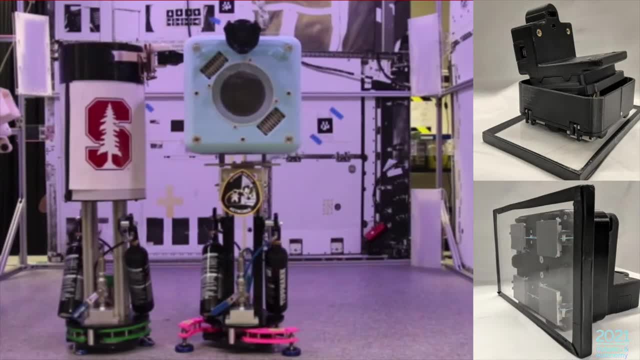 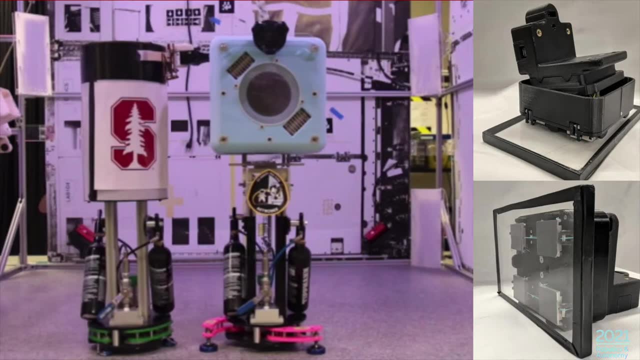 that we developed in our lab, as you can see here on the right. In addition, through a collaboration with NASA Ames and the Mars Kutkowski Group at Stanford, we're working on planning and control techniques to grasp and manipulate objects in space. Here I'm showing some tests at NASA Ames. 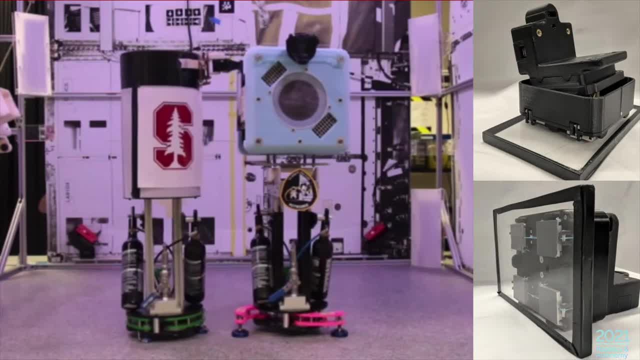 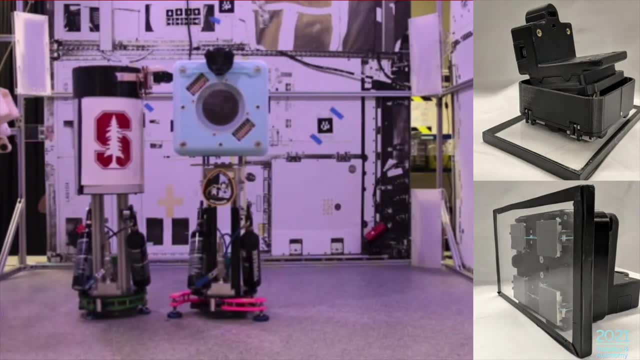 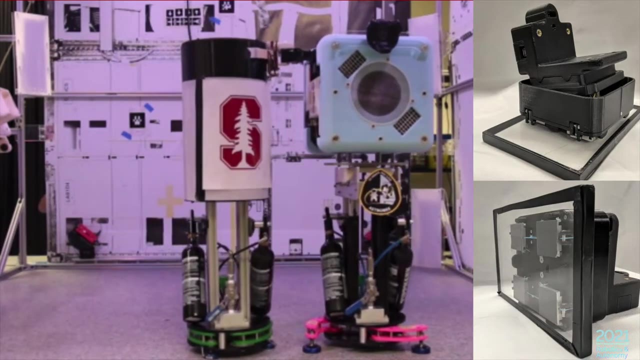 where zero gravity is emulated by using air bearings of a very flat granite table. The arms of the robot, the blue one that you see here- are equipped with gecko-inspired grippers. These grippers are equipped with pads that, by exploiting directionally-aligned micro-features. 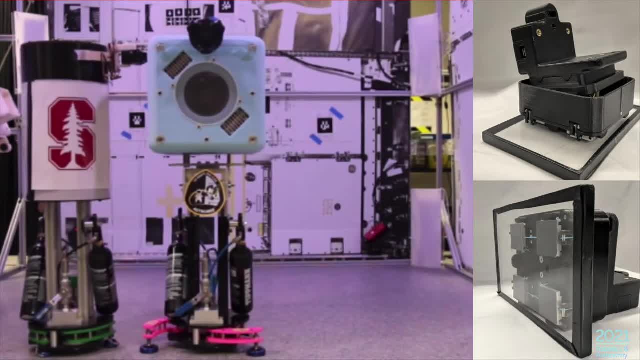 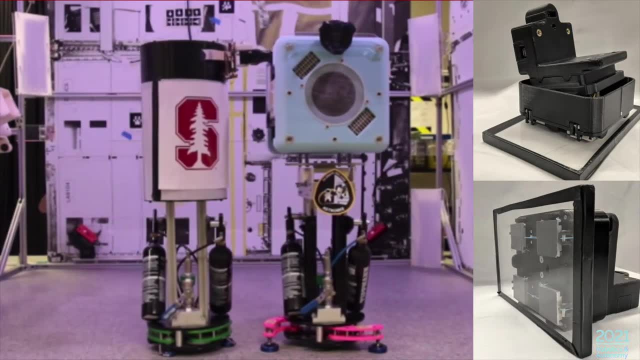 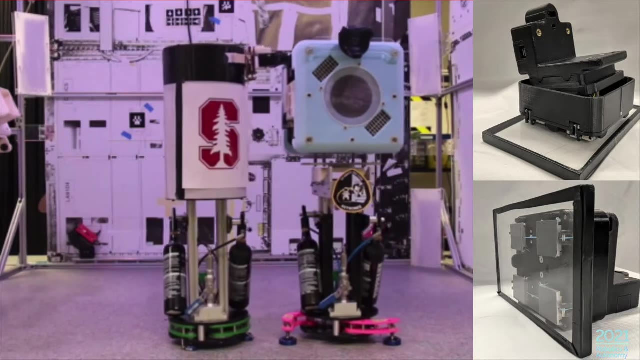 become adhesives When loaded in shear stress. a flat-qualified version of the gripper that you can see on the right has been sent to the International Space Station in 2019, and will be tested on the International Space Station in mid-April. So if you invite me again next year to this, 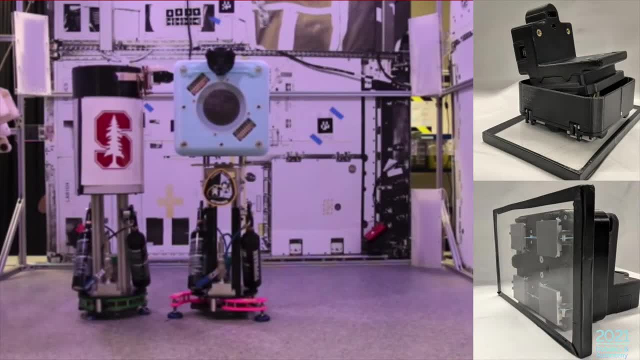 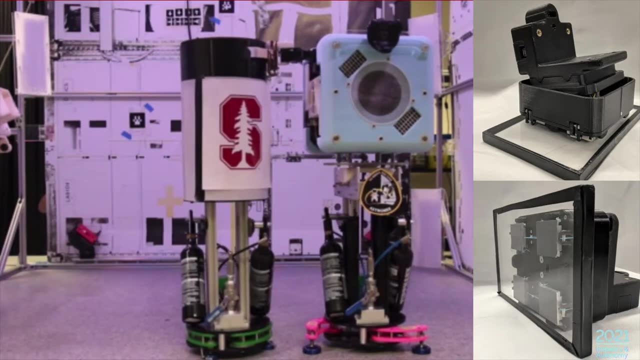 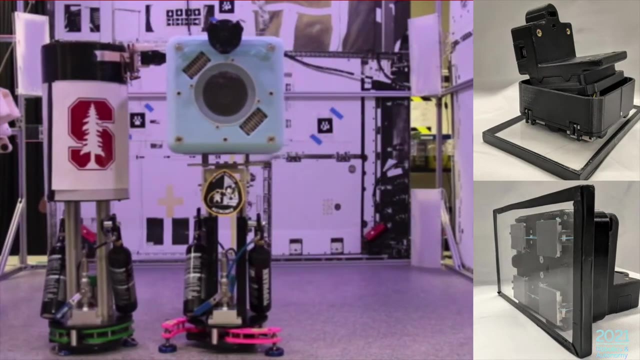 conference, I will be able to report on the results of these experiments in space, which is pretty exciting. Now, in all these applications, increasing the level of autonomy represents a major challenge due to the uncertainty of the environment coupled with the very often and sometimes stochastic 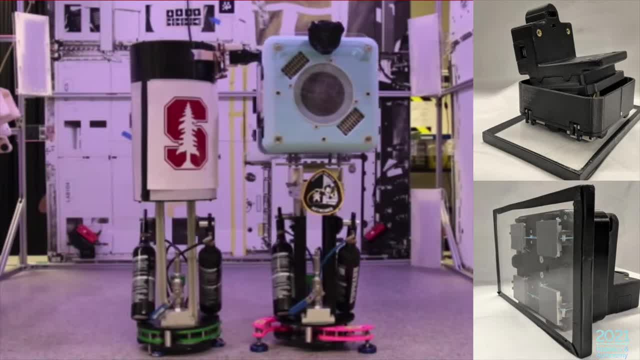 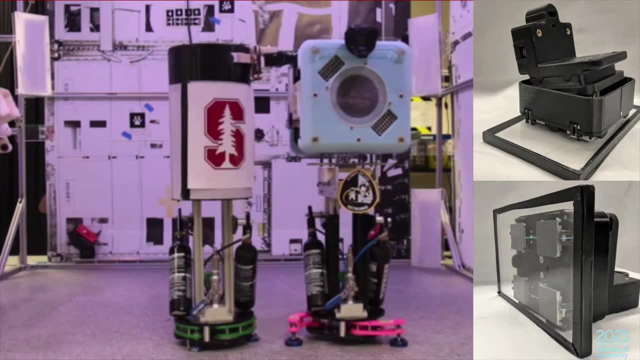 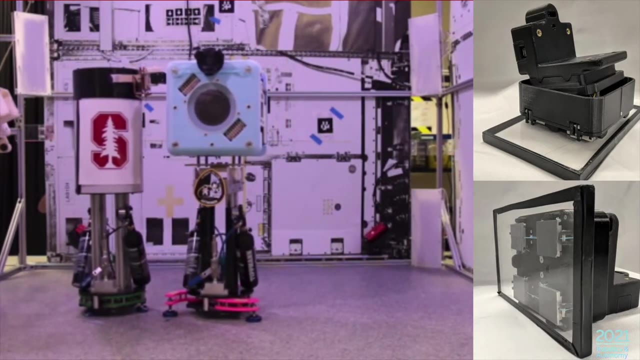 nature of the underlying dynamics of the systems. A very promising direction to tackle such a challenge is indeed to carefully blend techniques from machine learning and optimal control to harness the remarkable generality of the former and, at the same time, the sound guarantees of the latter. 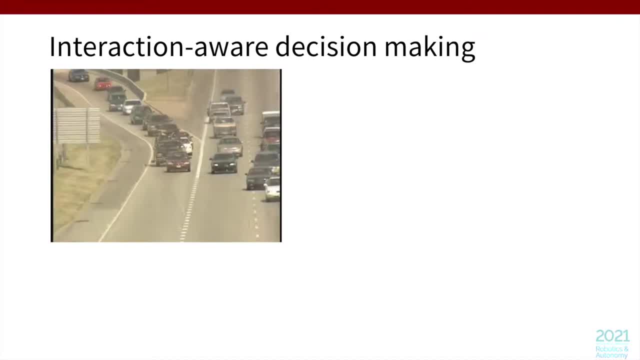 Safely and efficiently managing human-robot interactions represents another prime example of a setting that necessitates the principal blending of optimal control and machine learning techniques. In fact, modelling human behaviour is arguably best addressed via data-driven methods and, given the safety-critical nature that characterise human-robot, 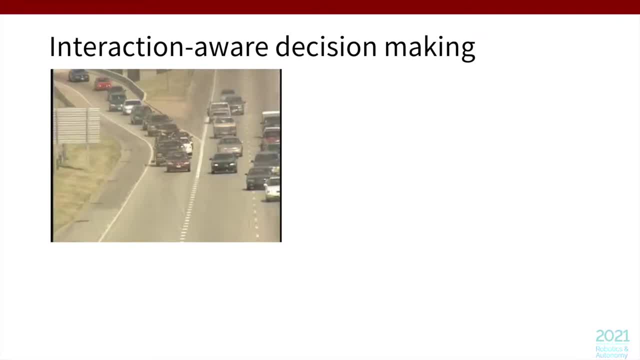 interactions. the control of the robot generally benefits from the principal inclusion of optimal control techniques. Indeed, the goal of this talk is to discuss my work on blending machine learning and optimal control techniques to achieve safe and efficient human-robot interactions By using autonomous driving. for the rest of this talk, 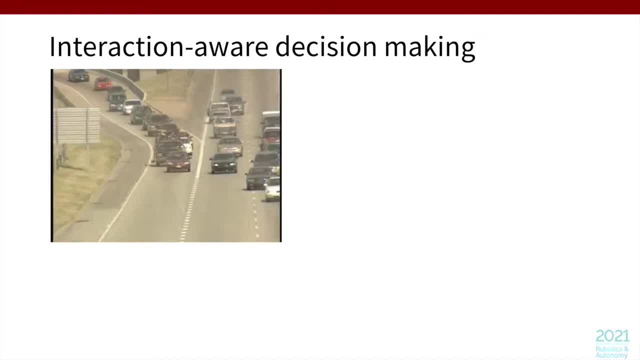 I'd like to start by introducing a few examples of how to do so. Driving indeed entails complex interactions. For example, in this video, I'm showing a setting whereby some vehicles are trying to merge onto the highway, other vehicles are just trying to go straight, And even though the overall intent of everyone 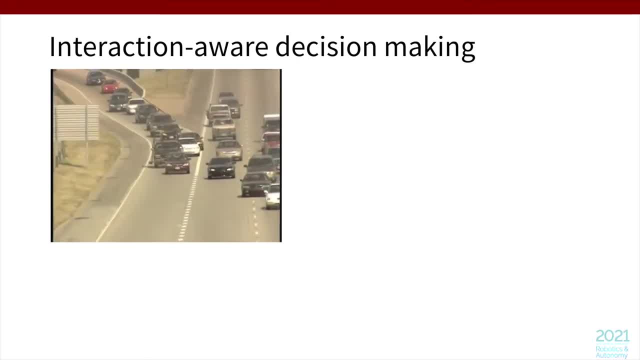 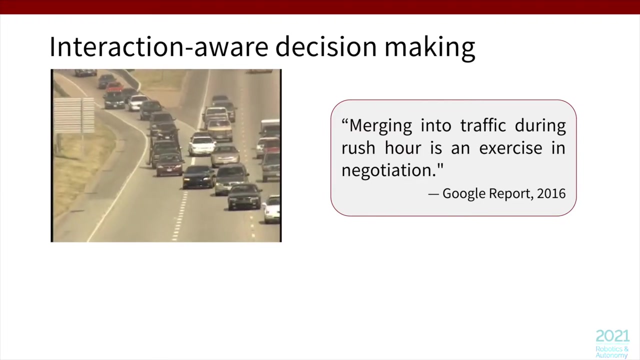 is pretty clear. some vehicles are trying to merge, some of the vehicles are just trying to go straight. the outcome of each interaction is highly uncertain, And it depends on a complex and sometimes even aggressive negotiation between and among the different agents. In other words, and I'd really like to mention this quote from a Google report- 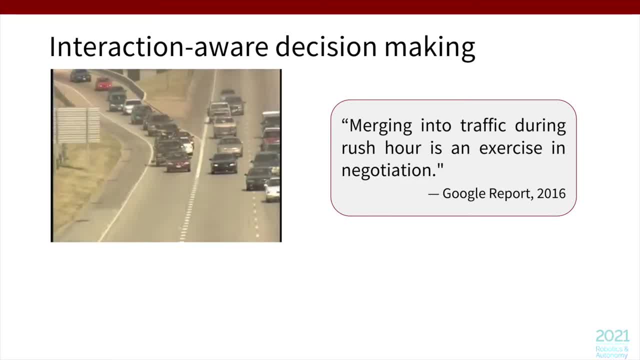 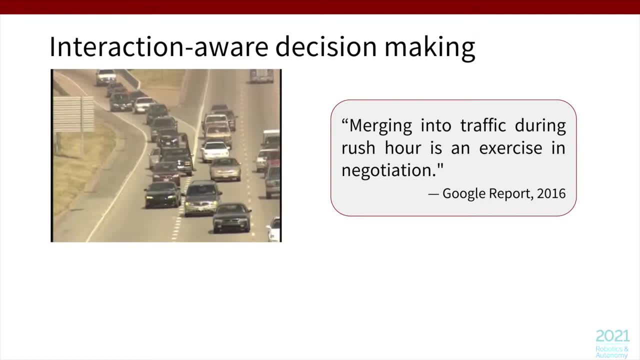 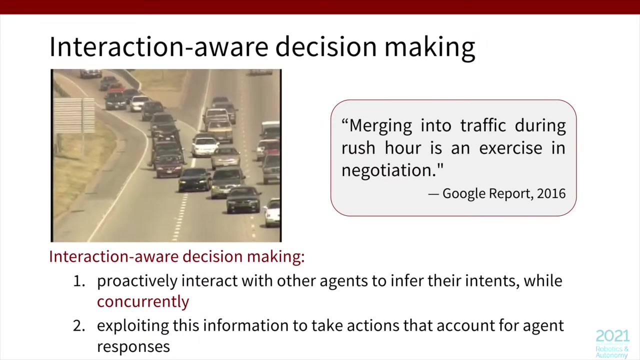 merging into traffic during rush hour is an exercise in negotiation, And autonomous cars, and robotic systems in general should be able to perform such negotiations for safe and efficient behaviour. In other words, robots, and particularly self-driving cars, should be able to perform interaction-aware decision-making, which refers to the 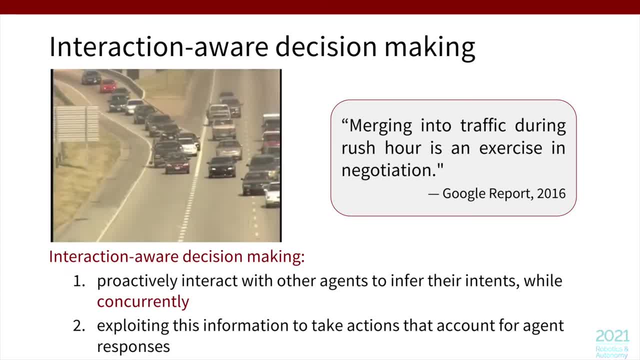 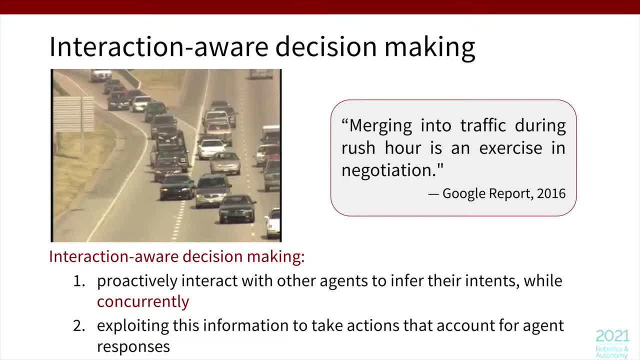 capability of proactively interacting with other agents to infer their intents, while concurrently exploiting this information to take actions that account for agent responses. Humans are decision-makers, so they're going to respond to the decisions of other agents- And I'm going to what the robot is doing- and it's imperative to account for these interactions. So, in order to 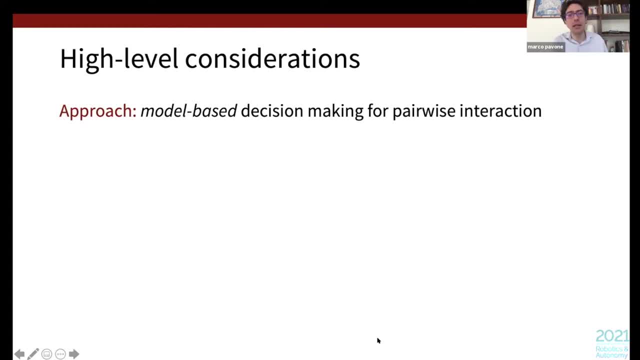 enable proactive decision making. one could follow either a model-based or a model-free approach. In my work, I advocate a model-based approach, whereby an understanding of the probabilistic structure of the interaction dynamics is used as the basis for policy construction. This is different from a typical model-free approach, whereby the 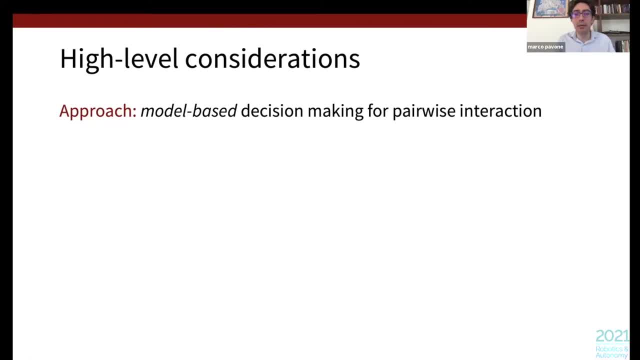 possible human actions and responses and the relative likelihoods are only implicitly accounted for in a policy that is directly learned from data, And the reason for advocating a model-based approach is that by decoupling the action-reaction responses from policy construction, one can achieve a level of transparency in a design. it is typically 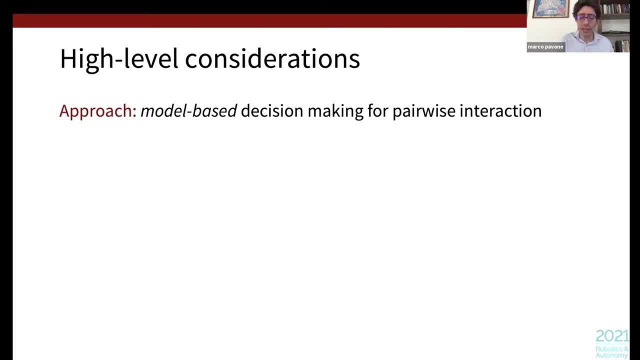 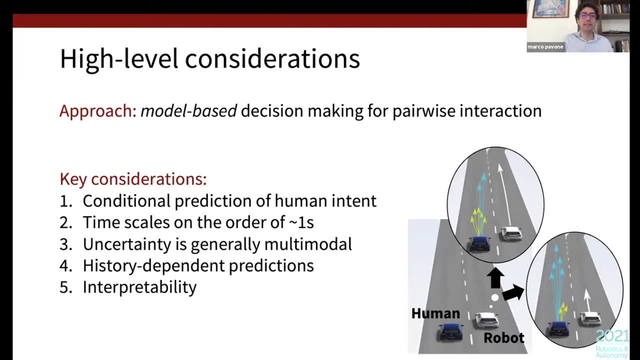 very difficult to achieve in a model-free approach. Now, the first step to enable a model-based approach to proactive decision making is to design a model that allows us to predict human behaviour and forecast the trajectory of the interaction environment. So we want to achieve ancanzlich. presence of a transportable platform in the model-based approach. offspring experts can also discuss an maybe some post-credit model-based approach and how every model-based protocol works here. In both cases, human behavior costs would also be a complication of β-shafsk and cf에게상을ism. 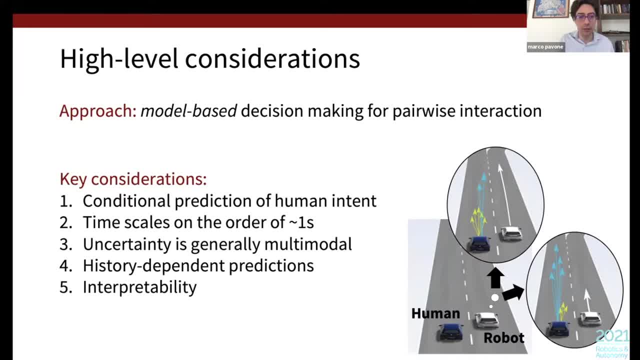 of every human agent on the road. So my work on devising a model for human behavior prediction is guided by five key considerations. The first one is that, from the point of view of decision-making, we're interested in reasoning about predictions of human intent. 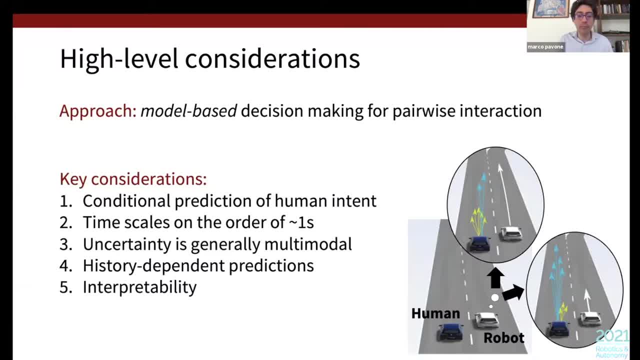 conditional on what a robot might do in the future. Second of all, in this setting we're targeting problems with a time scale on the order of one second. This is different from a traditional high-level decision-making that reasons in terms of macro actions. 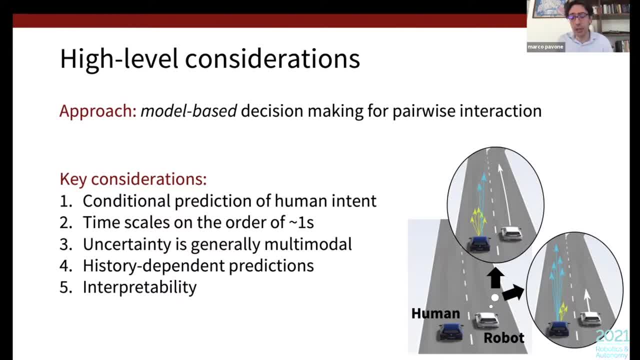 at the level of multiple seconds, And this is also different from low-level collision avoidance, where typically one reasons at a much higher frequency, say 100 hertz and beyond. So we're a little bit in a gray area between decision-making and the low-level control. 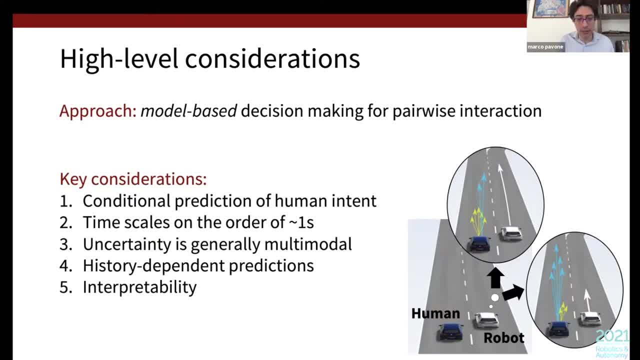 Third, at this level of the decision-making problem, uncertainty is generally multimodal, corresponding to drastically different futures for all the agents on the road. Consider, for example, the setting on the right-hand side whereby we have two vehicles, a robot-driven vehicle, 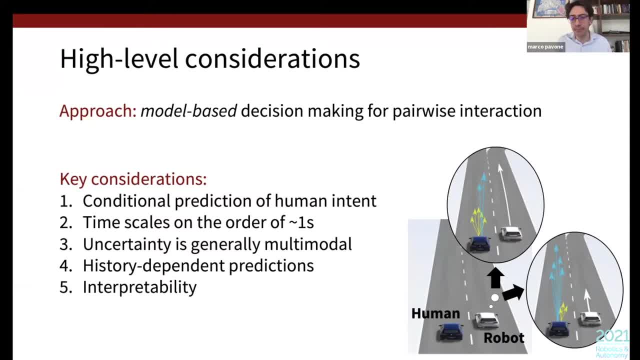 and a human-driven vehicle that are trying to swap lane. Now, if the robot is trying to swap lane, if the robot is trying to swap lane, if the robot were to accelerate as depicted by the long white arrow on top, the human-operated vehicle, the blue one. 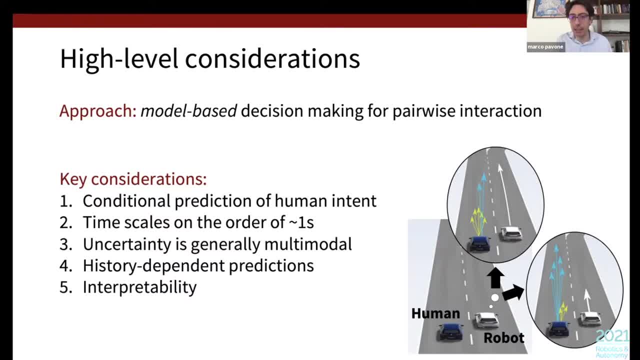 might either accelerate, as depicted by the blue arrows in the top, or might decelerate, as depicted by the yellow arrows, And this corresponds to two drastically different modes of a probability distribution that should be accounted for by the behavior prediction model. Fourth, it is important to account for history dependence. 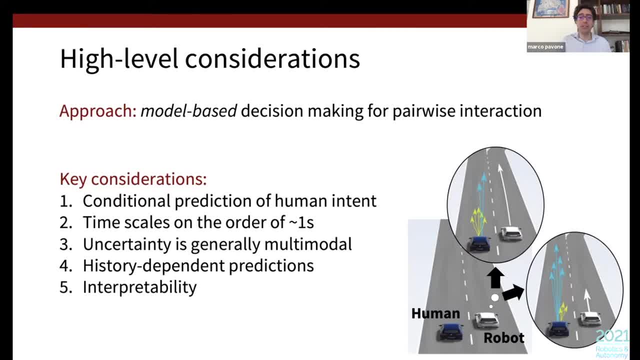 history of an interaction, to uncover latent behavior such as aggressiveness or alertness. And finally, of course, we want to have a framework as interpretable as possible to ease the bugging and to increase the level of confidence in these methodologies. 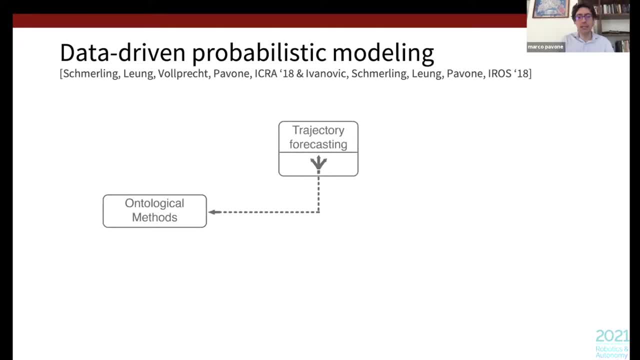 Now, in order to predict intent, there are one popular paradigm, which I refer to as ontological or theoretical. which I refer to as ontological or theoretical. but a theoretical approach requires very much of a혀 theory in mind, entails postulating some structure. 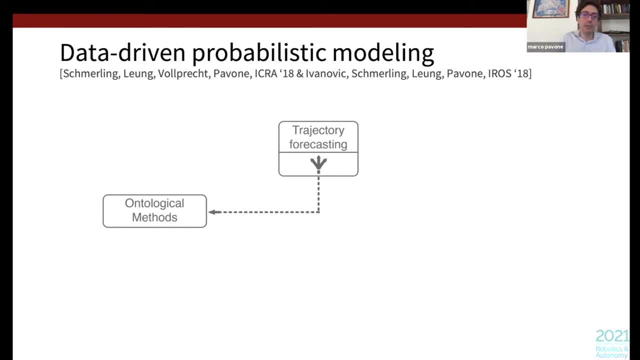 on how humans make their own decisions, For example, in terms of a cost function that we postulate a human is trying to optimize in order to compute its driving actions. And then the idea is to learn that cost function from data. and once you have learned that cost function, 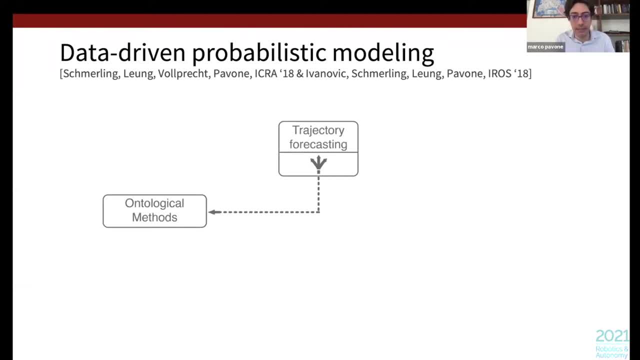 one can predict the next action by computing the action that minimizes such cost function. Now, the point here is that such a theory of mind approach is sometimes difficult to reconcile with how humans really operate. Humans typically, are neither cooperative nor adversarial. and such a fascinant behavior. 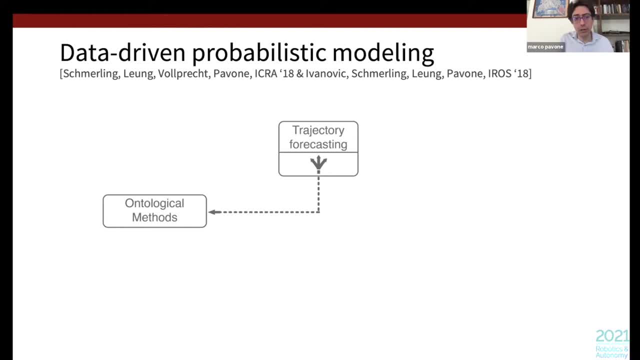 is difficult to reconcile with an ontological or theory of mind approach, which is ultimately rooted in game theory. So in my lab we have been considering a completely different approach that I refer to as phenomenological, And the key research question here is: can we learn action distributions directly from? 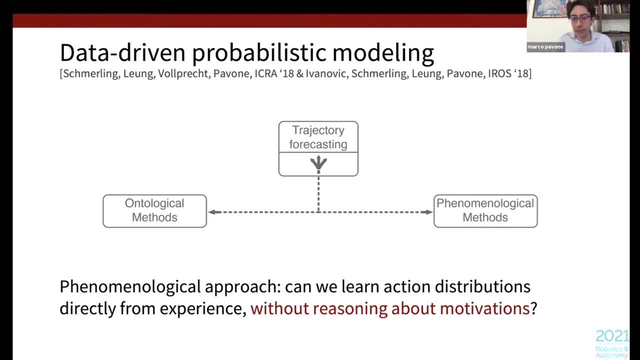 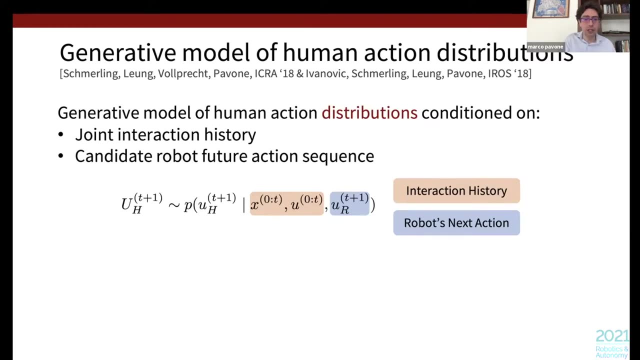 experience, without reasoning about underlying motivations, So basically without placing or postulating assumptions on how humans make their own reasoning Explicitly. there has been a lot of work in the past few years, For instance on genetic modeling, that is, on how to predict the future. 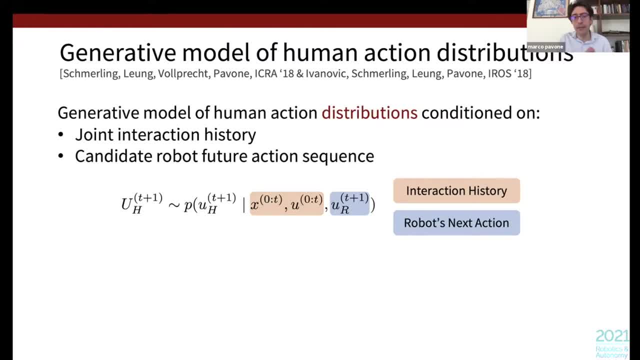 Where our work differs from the norm is that we are interested in predicting future behavior not only as a function of past observation, but we also want to reason in terms of how a human might respond to a possible candidate future of an action. Specifically, 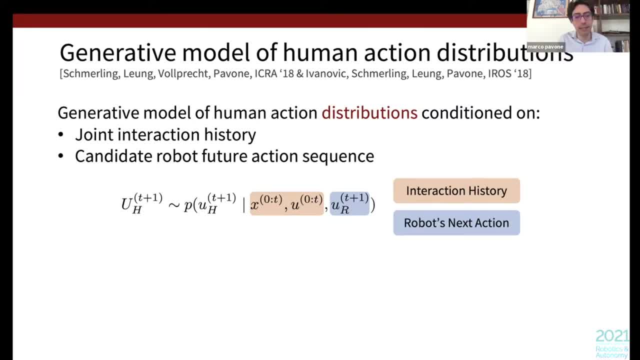 learn is a probability distribution with respect to the next control action of a human depicted as u h t plus one. in this talk, subscript h stands for human. t plus one denotes the next step. so we want to learn the probability that a human will enact at the next time step a given control action. u. 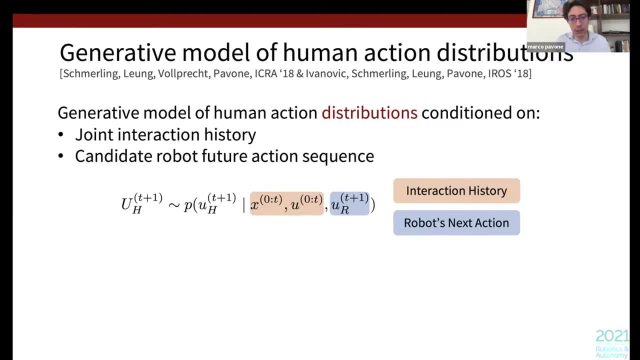 conditional on the history of the interaction x and u, so this could be, for example, relative positions or relative speeds in the previous t time steps. comma, and this is the next one, is the element in blue, critically. the next also conditional on the next robot action and here the 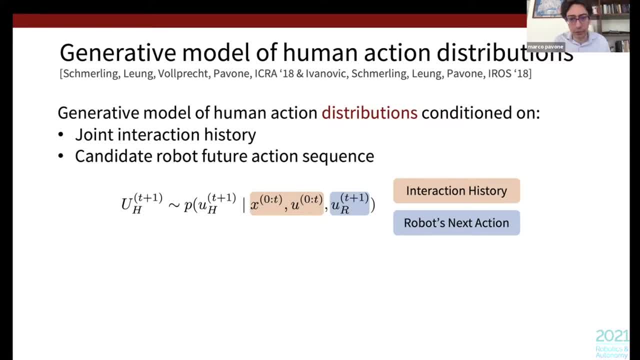 idea is that the conditioning on the history of an interaction allow us to uncover latent behavior such as aggressiveness, while conditioning also on the future candidate robot actions allow us to capture the interactive aspect of an interaction. so in practice, we use a conditional variation autoencoder model to learn. 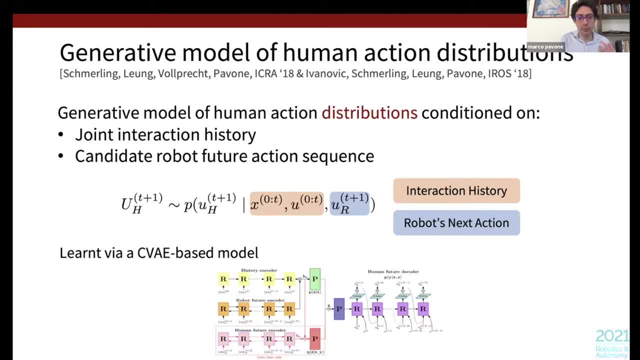 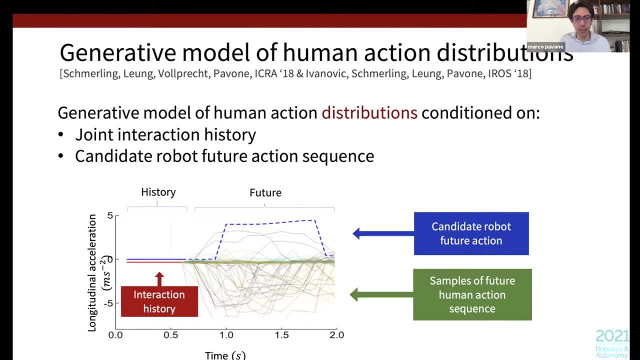 such a distribution, and the way that, then, we use this model is as follows. here we consider the setting whereby we are trying to predict longitudinal acceleration. on the x-axis, we have time. on the y-axis, we have longitudinal acceleration, a solid line that depicts quantities that have happened. 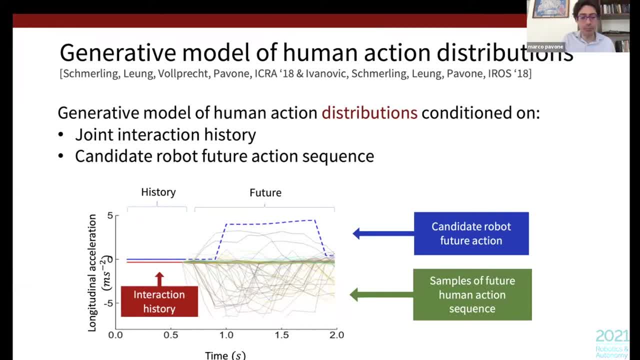 in the past. so we see here that in the first 0.7 seconds both the robots represented by blue line and the human represented by red line were going at constant speed, so zero longitudinal acceleration. and then at 0.7 second time we probe the model to. 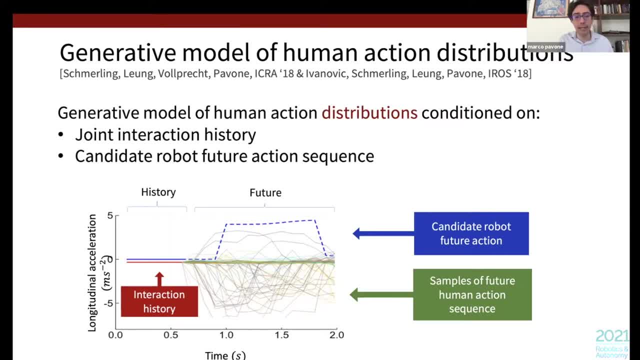 ask the following equation: if the robot were to enact a action sequence whereby it first accelerates, then it costs at a constant speed, and actually at a constant acceleration, and then it decelerates, what will be the possible reactions from a human? and this is that's how we basically 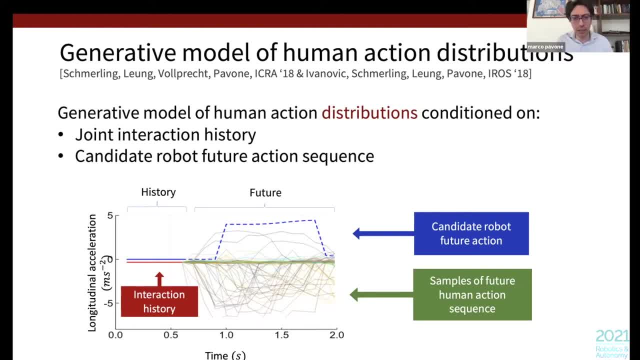 sample, the genetic model and on the and all the lines that you see are all potentially possible responses by the human. you see that our model in this case predicts that in most cases the human would decelerate if the robot were to accelerate, which is kind of reasonable. but you also have some predicted trajectories where we 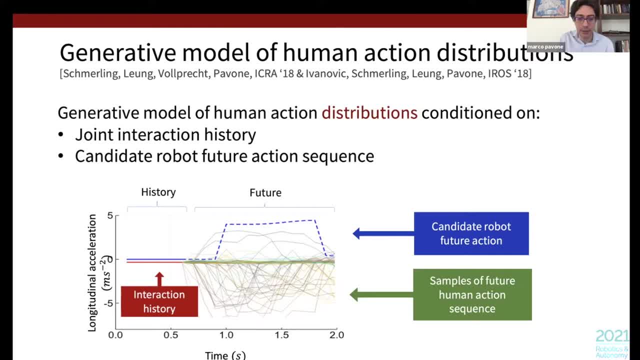 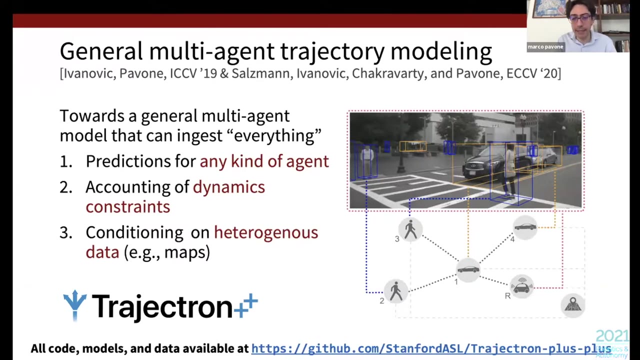 we believe that actually the human might accelerate. so basically we obtain, by sampling the genetic model that we have learned from data, a bunch of potential responses to a candidate robot, future action sequence depicted again in the dashed blue. so we have extended this model to be capable of considering, as a conditioning, variables. 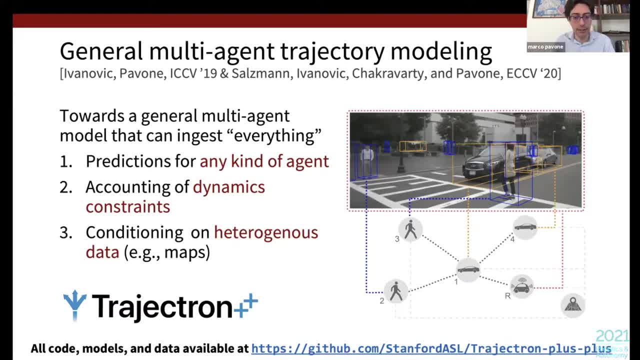 a vast set of heterogeneous data, for example, dynamical information about the different agents- obviously, human moves in a way that is different from a car or a bike. information about a map, for example in terms of road boundaries or crosswalks, and even human silhouettes, which is quite important. 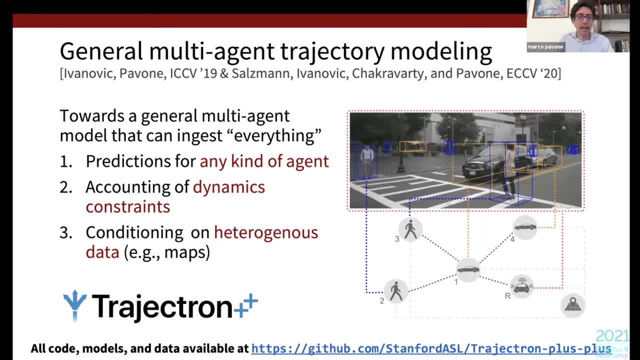 in order to predict the pedestrian behavior. the end result is a trajectory from plus plus, which is a generative trajectory modeling framework that is capable of explicitly reasoning about the agent dynamics and encoding a vast array of heterogeneous information as conditioning variables. all the code, models and data is available on our github page. 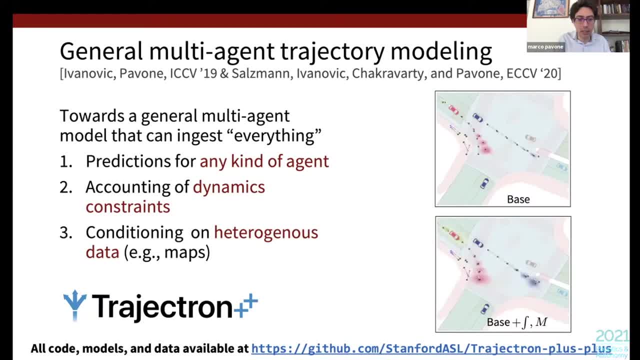 so we tested this model on the number of data sets by achieving state-of-the-art performance relative to both deterministic trajectory forecasting models and the general trajectory forecasting models. So I defer you to the papers that I mentioned in this slide if you're interested in learning more about the benchmarking. 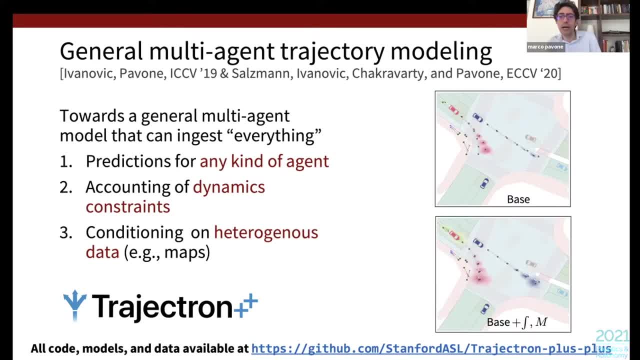 that we've done Here in this slide. I just want to show you how important it is to reason about the dynamics and the maps as conditioning variables to predict future actions of the different human agents on the road, For example. let's focus on so specifically. let's. 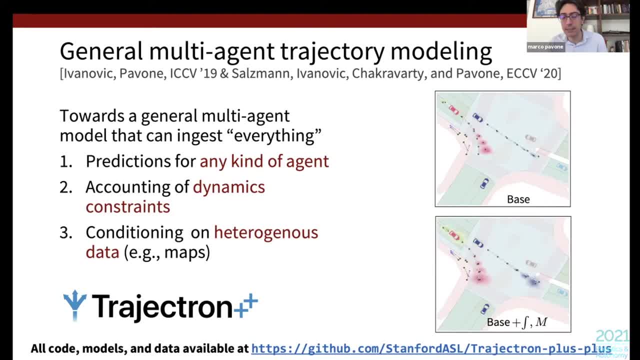 focus on the picture on the top right, So we want to predict the future trajectory of the red vehicle. on the top left, The white line is the ground truth trajectory. The blobs- the red blobs, are basically our predictions, by using Trajectron++ in its base implementation. 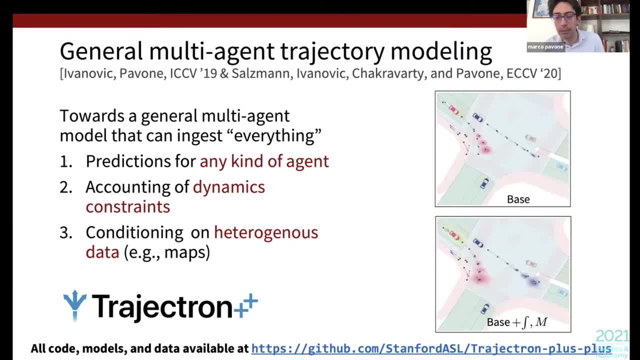 without taking into account the dynamics and map information. As you can see, here in our prediction we are undershooting the ground truth and, even worse, the ellipses. basically those are our confidence. ellipses barely intersects with the ground truth, which basically means that not only 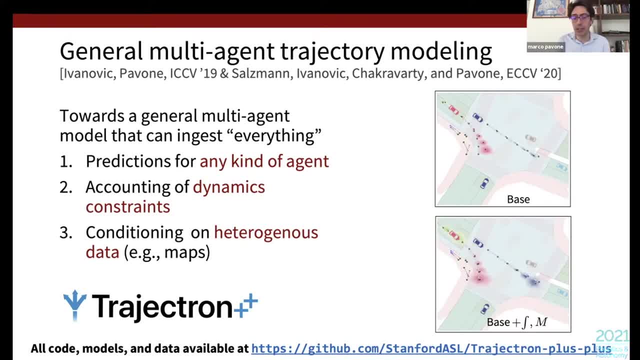 we are undershooting the ground truth trajectory, but we are also overconfident. At the bottom. we see that once we actually augment the model to be capable of accounting for dynamics and map information, then the forecasted trajectory, again represented by these red blobs, 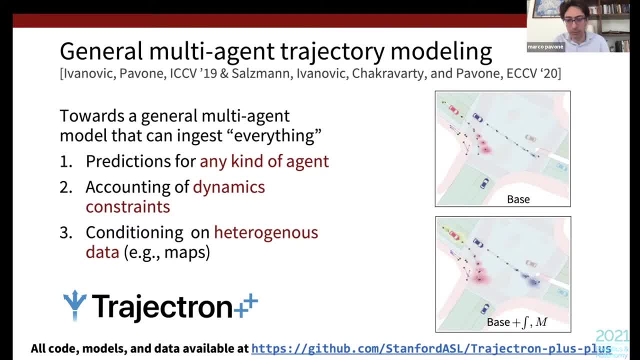 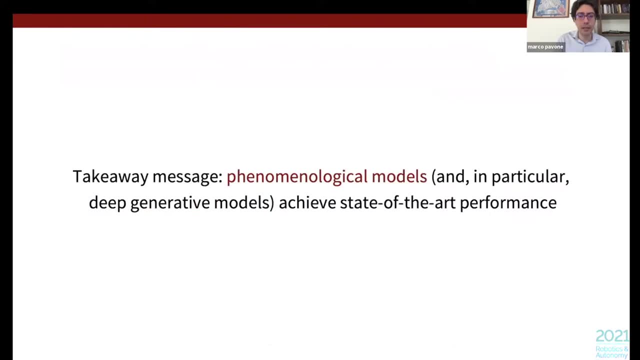 will change. The predictions are probabilistic, align very nicely with the ground truth. So this is just to show how actually accounting for these additional layers of conditioning variables is very important in order to better calibrate predictions. Now the takeaway message for this first part of the talk. 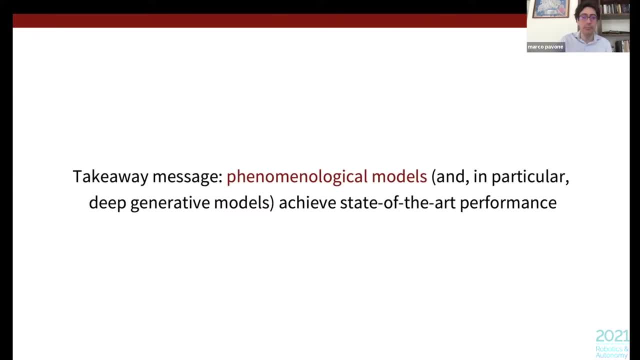 is that the phenomenological models, and in particular, deep generative models, achieve state-of-the-art performance. When we started this research about three years, two years ago, ontological models were the de facto standard in this setting, But now phenomenological models, partly because of our research. 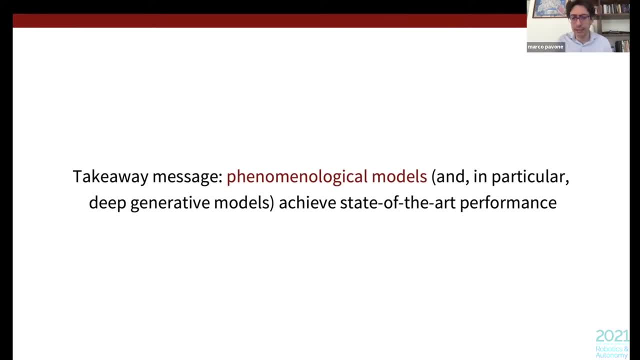 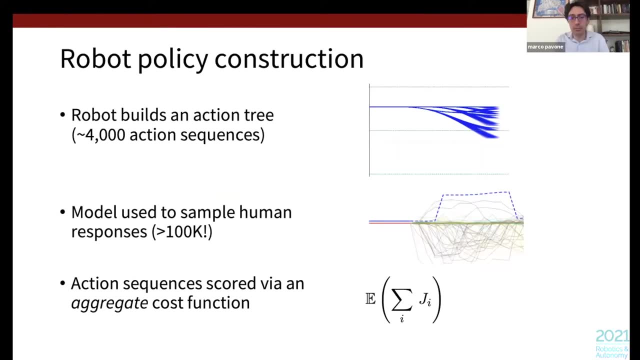 are becoming the tool of choice for this type of applications. Now in my lab, we are interested in decision making, So how do we then use these models for the purposes of decision making? So the way we use these models is as follows. 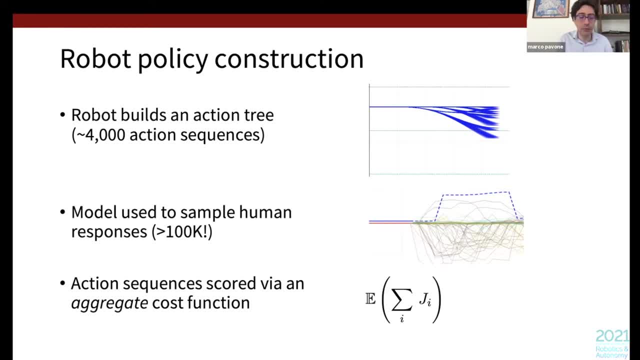 We build a set of motion derivatives, Basically candidate trajectories, that differ in terms of the longitudinal acceleration profile and the lateral acceleration profile. In actuality, we consider about 4,000 action sequences And then, for each one, we consider each trajectory. 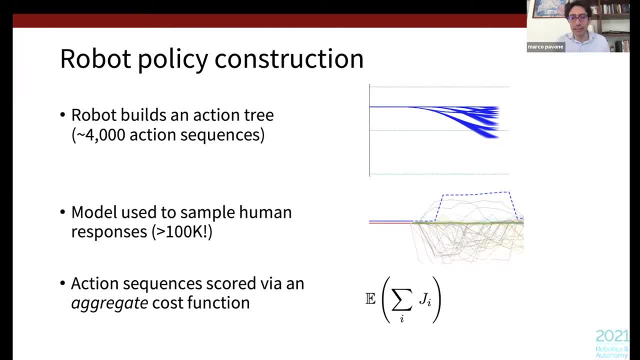 as a conditioning variable for the trajectory forecasting module and for each trajectory. we ask the following question: If we were to enact this trajectory, what would be the, what will be the possible human responses? That's exactly what the trajectory from PLUSPLUS enables us to answer. So, for each trajectory, by probing the CVAE model that I mentioned before. 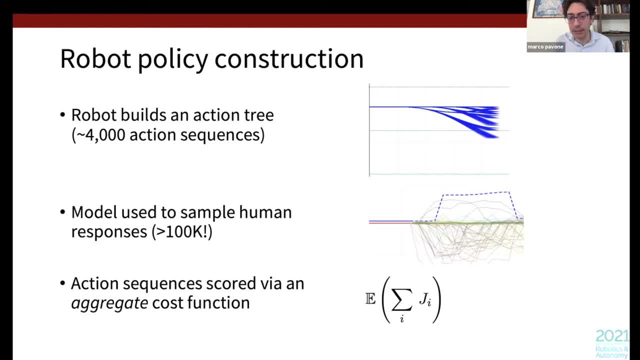 we obtain a bunch of possible reactions from other humans on the road And then we score each motion primitive along with the family of reactions from the humans, by using an aggregate cost function. This is quite standard. We pick the best one and then we drive the first chunk of it, and then we 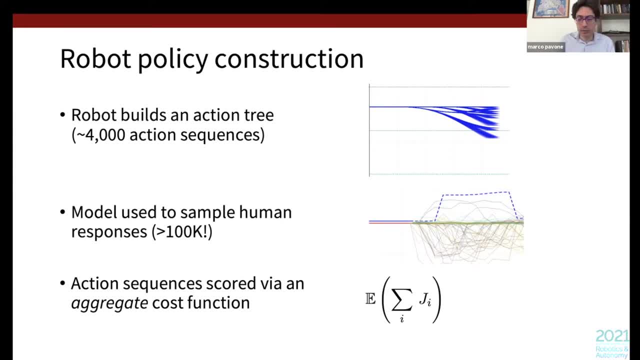 replant. Now, this process is highly parallel, So by leveraging basically an implementation in GPU, we can run each computation cycle in the order of about 1 to 200 milliseconds, so at about 5 hertz, which is a lot. 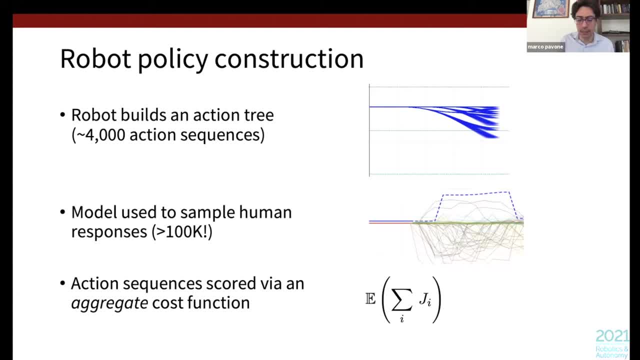 Now, an important point that I want to make here is that when we predict the future trajectories for all the other agents on the road, those predictions are probabilistic, They're stochastic And actually we have distributional information about the responses from each human. So in our 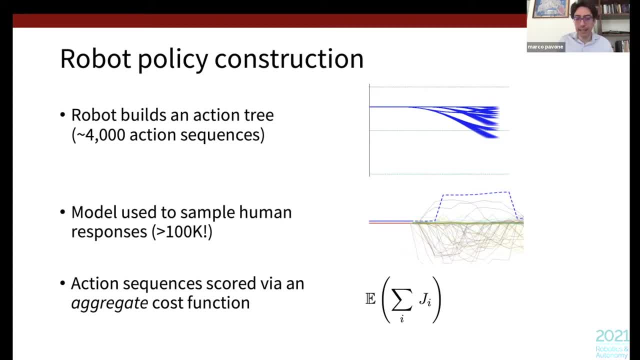 work. we consider the average of an aggregate cost function, where the average is taken with respect to all possible human responses. But since we have distributional information, you might consider: well, why don't you also account for what happens in the tail? So why don't you have a more explicit 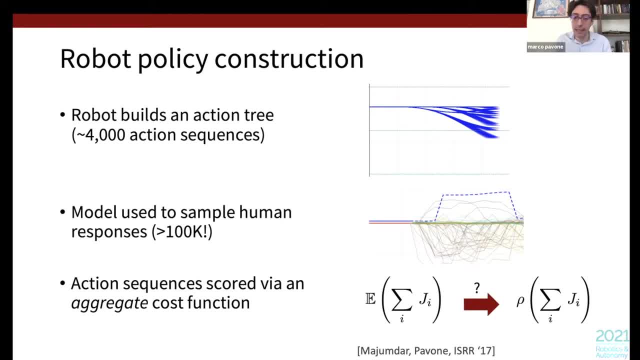 accounting of events of low probability and detrimental outcome, which mathematically would mean to swap the expected value operator E with the risk measure rho, whose purpose is the latter, but is exactly to put more emphasis on what happens in the tail. So how to assess risk? 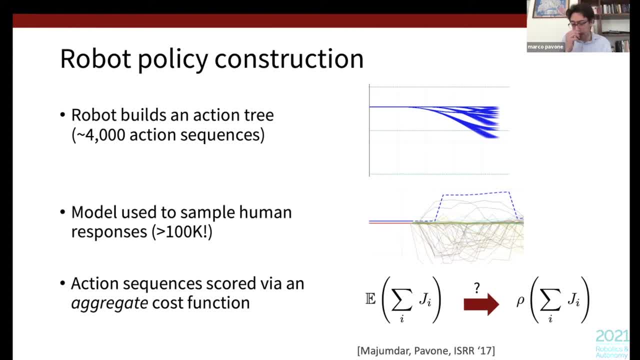 from robotics. application is a fascinating topic and also a difficult one, both because of computational reasons and also because of well-posed reasons. So coming up with a risk measure that makes sense is not that easy. In the interest of time, I won't go into these. 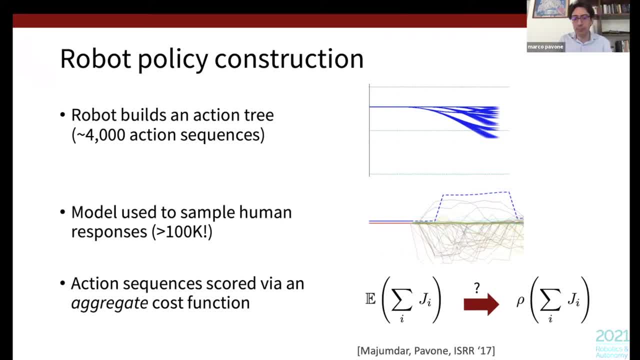 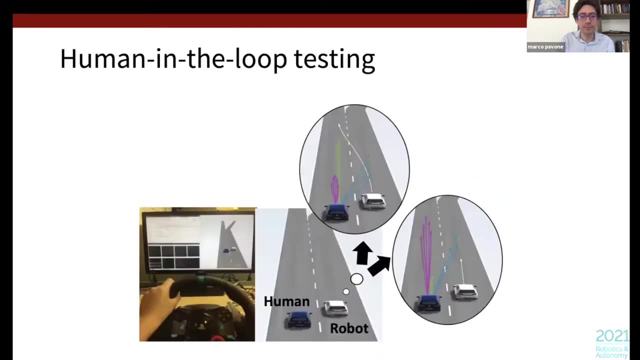 details, but I refer you to sort of a position paper that I wrote with a former postdoc in my lab, Annie Majugmat, now a faculty at Princeton. So it's basically a position paper about how we think people should think about risk in a robotics context. So, moving on, how does all of this work? 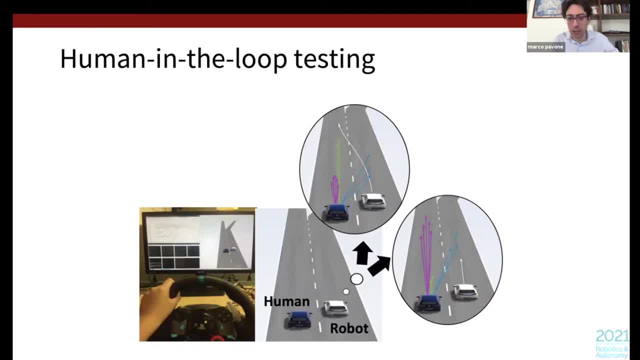 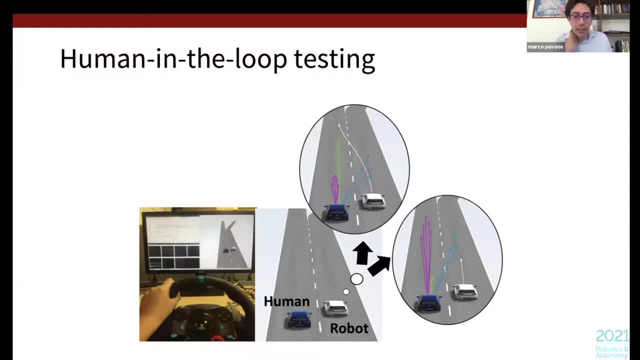 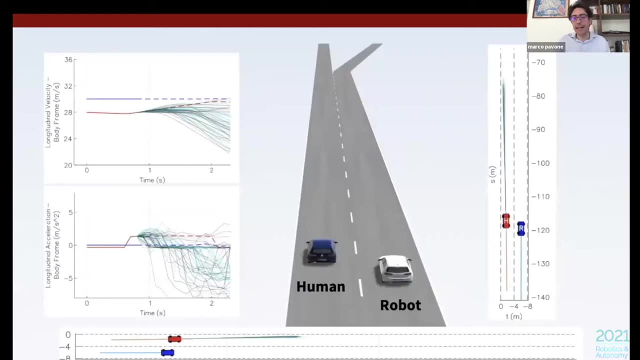 drives in simulation, in a variety of interactive driving scenarios, alongside a robotic vehicle. That is, a vehicle that is driven by using our algorithms, And here I'm showing an example of the simulations whereby, again, the task is a traffic weaving task. This is the recurring example. 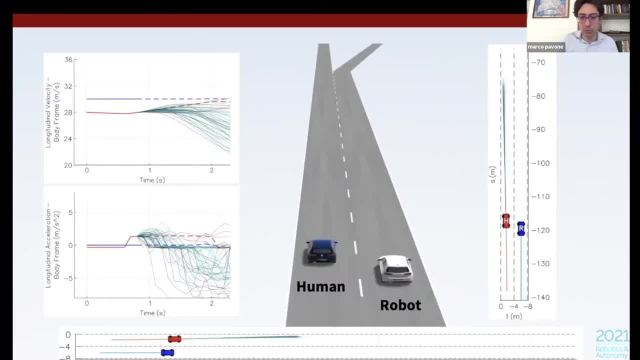 in this talk, Specifically the robotic vehicle, the white one, and the human-driven vehicle. so the vehicle driven by the student in our human-in-the-loop simulations have to swap lane before the road works On the left-hand side. the video is going to show you predictions in terms of longitudinal 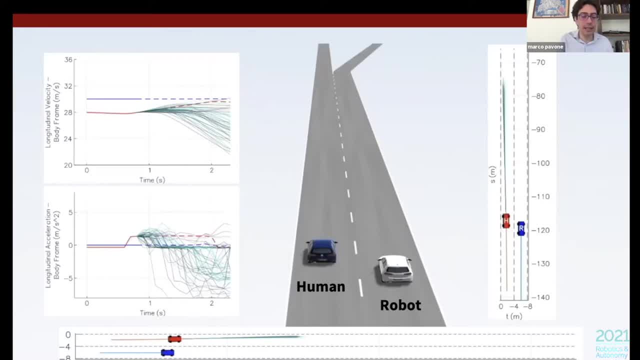 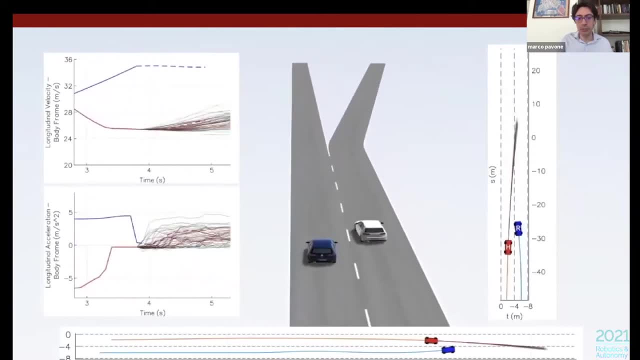 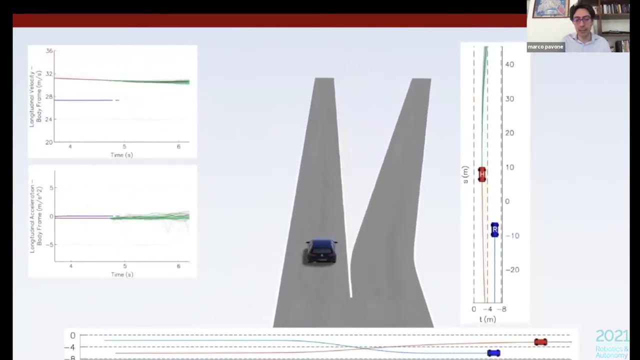 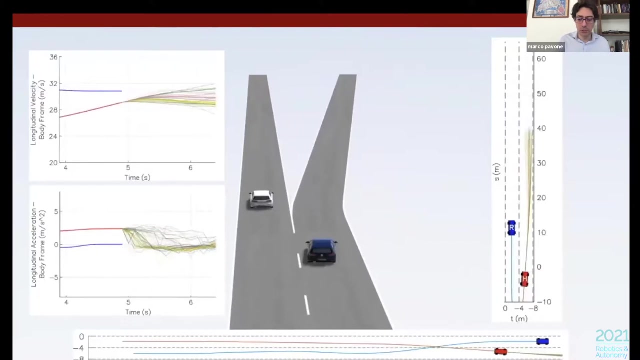 velocity and longitudinal acceleration for a given candidate robot action sequence. So here you can see that some interesting behaviors emerge, like, for example, the robotic vehicle- the white one- nudges a little bit on the other lane in order to disambiguate intent of the human-operated vehicle, and that the interaction is quite seamless, which is great. 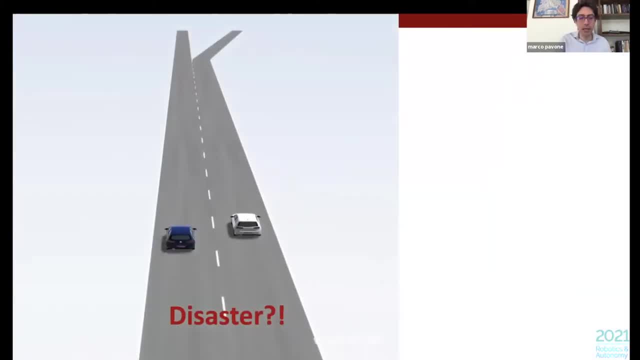 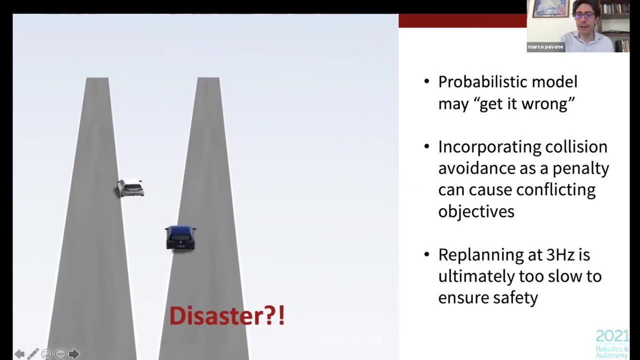 until disaster happens. So this is a case whereby the human- so the student- drives in a way that defies our expectations. it decides to swerve into the robotic vehicle and a collision happens. Now the point I want to make here is that, to some extent, 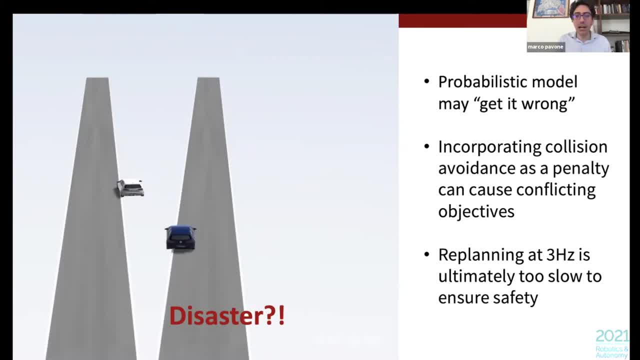 these bad cases are unavoidable, at least with the framework that I have developed so far. First of all, probabilistic models for trajectory forecasting, even sophisticated ones like the one that I presented, are still probabilistic, so sometimes we might guess it wrong. 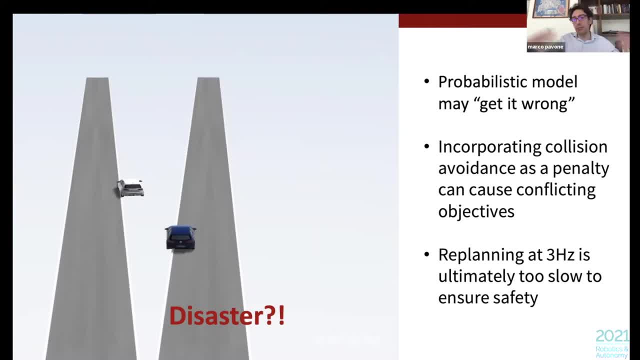 As in the case of us humans, when we drive we make a lot of predictions about what other people will do around us Rarely, but sometimes it happens that we guess it's wrong and there is pretty much nothing we can do about it. 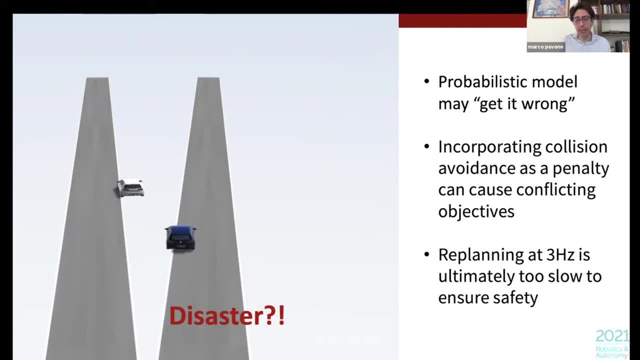 Second of all, at this level of the decision-making hierarchy, collision avoidance is typically incorporated as a penalty function amidst many other different penalty functions. This can cause conflicting objectives When you have such complicated aggregate cost functions. sometimes some of the different penalty functions might create conflict. 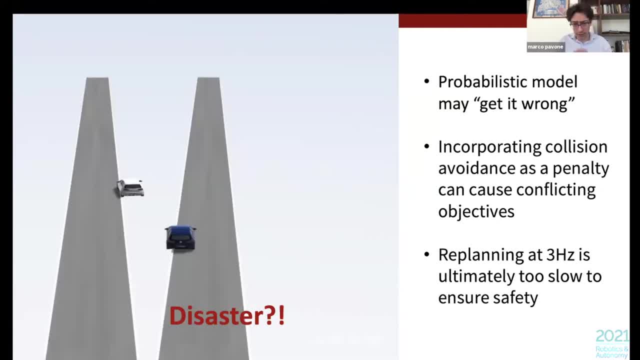 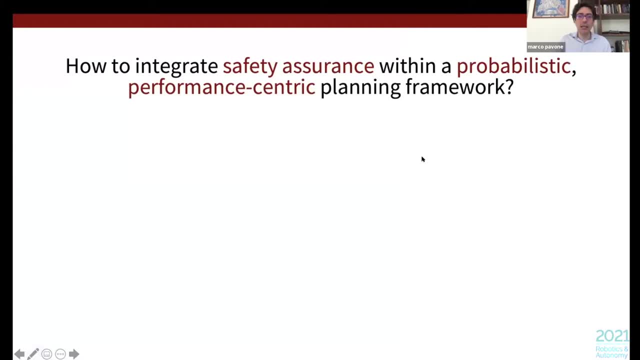 objectives. And finally, reprimand at three to five hertz is ultimately too slow to ensure safety. So this points to a key challenge in the field of safety-critical decision-making for autonomous systems. Specifically, how do we integrate safety assurance within a probabilistic 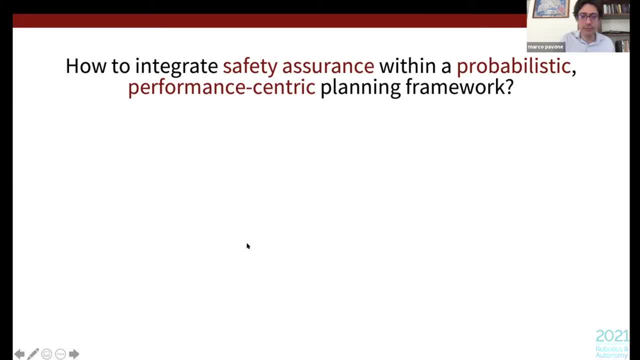 performance-centric planning framework. Specifically, here I'm showing a conceptual plot of a safety versus efficiency. The key point is that high-level decision-making algorithms typically reason probabilistically in order to promote efficiency at the cost of safety. So typically, high-level planners in the blue blob are highly efficient. 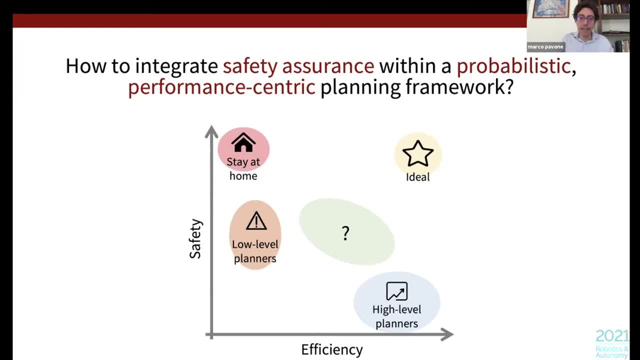 but sometimes they're not very safe. On the other hand, low-level planners typically reason adversarial or pessimistically with respect to the behavior of the other agents in order to ensure safety at the cost of efficiency, meaning you might stop very frequently in order to avoid a collision. 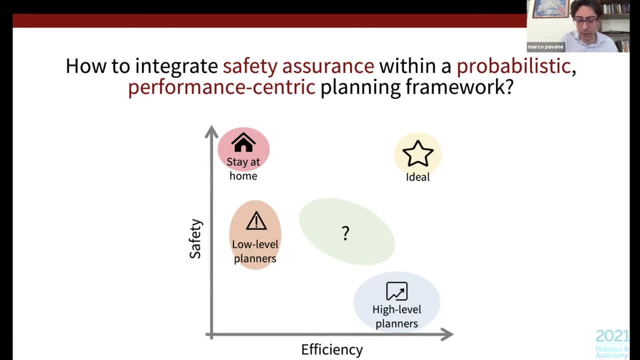 Safe behavior, but from a mobility standpoint not very useful. Ideally, you would like to be in the position denoted by the yellow star, So you might be maximally safe and maximally efficient. More realistically, we want to find a way to carefully. 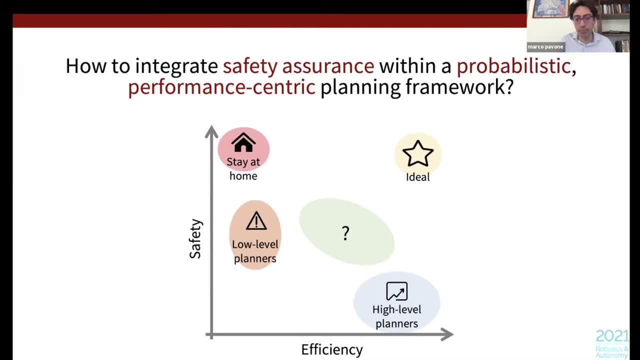 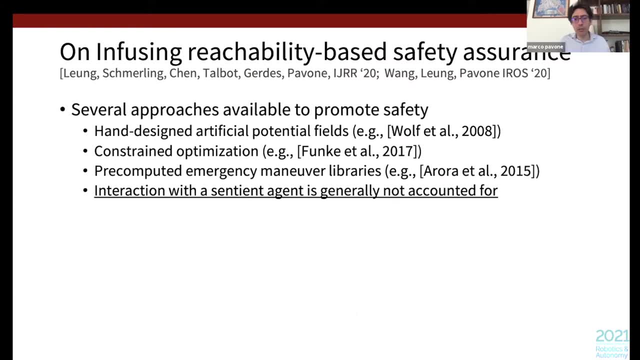 determine the trade-off between the safety and efficiency of low-level planners and probabilistic high-level planners respectively. From a more technical standpoint, I would say that the problem of how to glue probabilistic high-level decision-making with low-level collision avoidance has been largely overlooked in the academic. 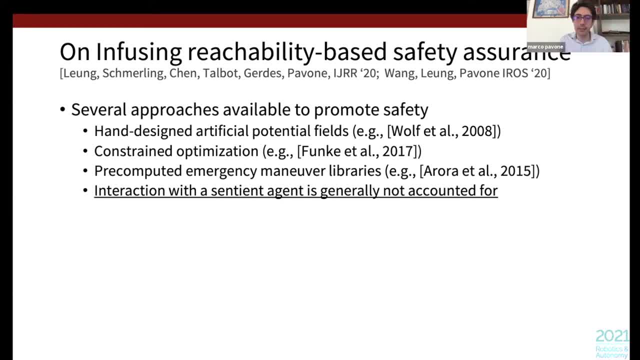 community. A lot of people working on high-level decision-making, a lot of people working on low-level collision avoidance. but how to glue these different layers of the autonomy stack? relying on drastically different assumptions on how the world behaves, is oftentimes a leap of faith. 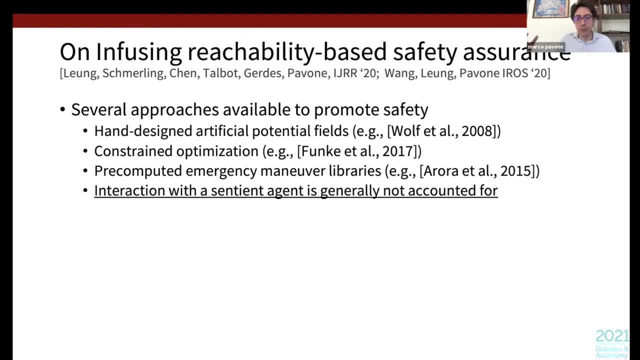 So what I'm going to do next is to show our solution to glue these different layers of the autonomy stack in a way that is as seamless as possible. I will first start by talking about how we design a low-level collision avoidance algorithm. that is more. 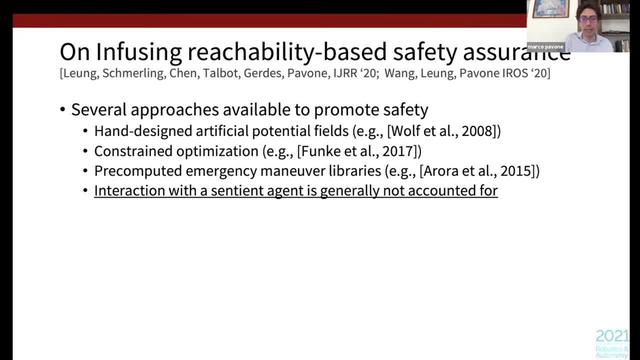 attuned to be blended with the high-level decision-making, and then I will present the full control and decision-making stack. Specifically, in order to enable collision avoidance, there have been a number of methods that have been proposed in the past, like, for example: 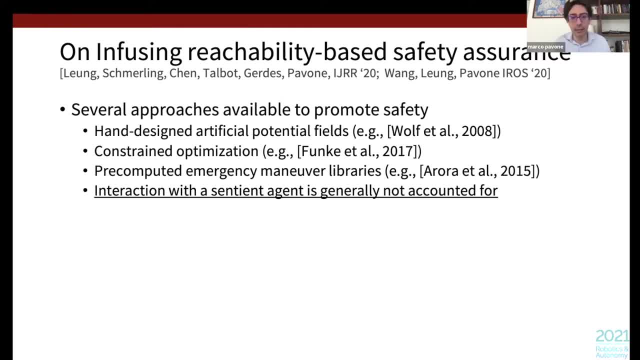 artificial potential fields, constraint optimization, pre-computing, emergency maneuver, libraries, and so on and so forth. But, critically, in all these methods they do not account for the fact that we are interacting with a sentient agent, an agent that is a decision-maker and is going to respond to what we do, And thus they are difficult to blend. 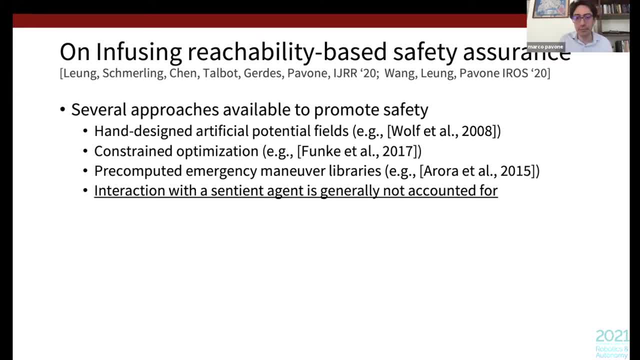 and merge with a decision-making module that is striving for efficiency through probabilistic reasoning. So what we do in our work in order to reason about interactions at the lower level of decision-making hierarchy is to embrace the tools of Hamilton-Jakoby reachability. 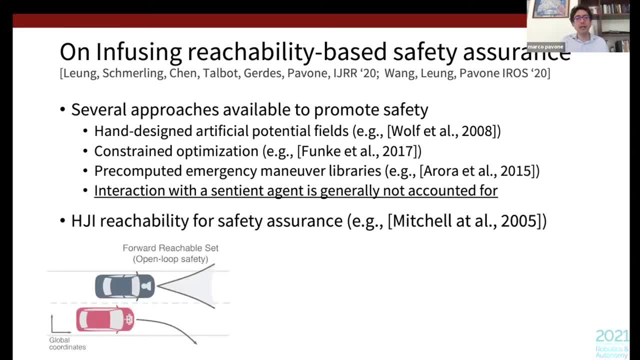 Now, reachability is often discussed in a forward open-loop sense, whereby, for example, the dynamics of the blue vehicle, the human-operated vehicle, are forward propagated in time for a couple of seconds, say, and then we treat the resulting set of possible positions where, 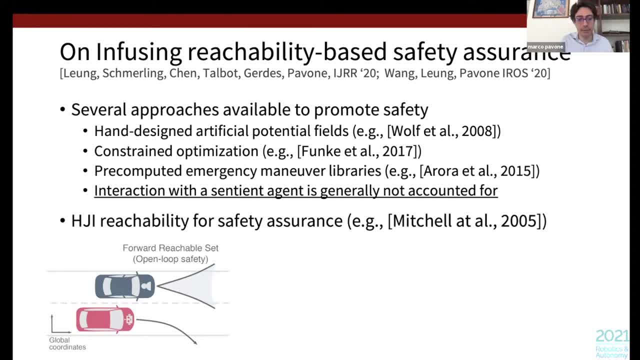 the human blue vehicle could be, in the next couple of seconds, as effectively an obstacle. And then for the robotic vehicle, the red one, we want to plan trajectories that do not intersect with that reachable set. Now, this style of reasoning is typically too conservative to be. 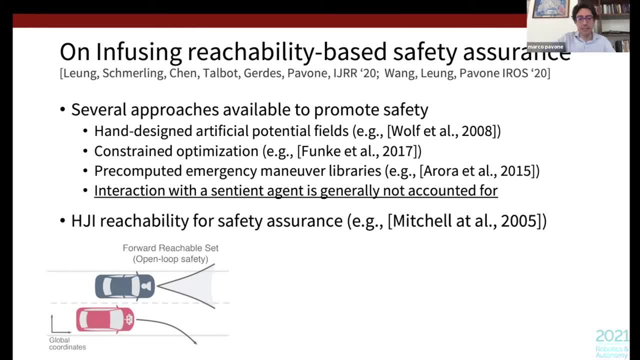 useful in practice. If you propagate for two, three seconds, basically, the reachable set is so large that there is no space for the robotic vehicle to plan a feasible trajectory. So what we do in our work is to embrace the tools of Hamilton-Jakoby reachability. So what we do in our work is to embrace the 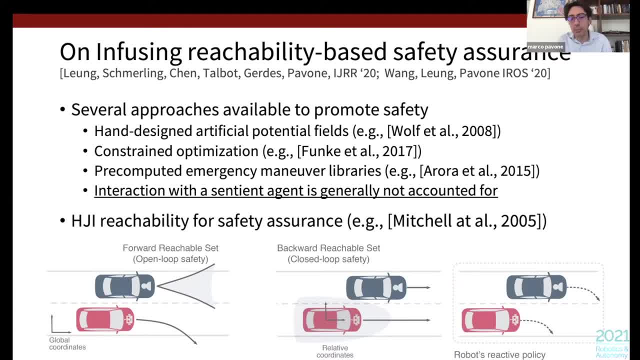 notion of a backward reachability, whereby the joint dynamics of the robotic vehicle and the human-operated vehicle are propagated backward in time in order to account for their interaction. The resulting set is referred to as a backward reachable set and encodes the notion of those relative states. you do not want to be in because, whatever the robot might try to, 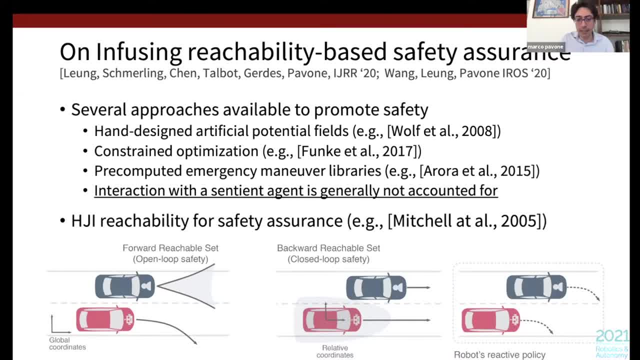 do to avoid a collision. there exists a control for a human that might lead to a collision. In very practical terms, I would claim that the way that I drive my motorbike is different from the way that I drive my car. Specifically, when I drive my motorbike, I'm very careful not to put 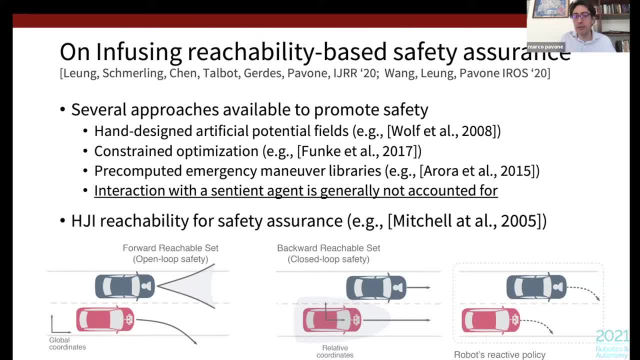 myself in a situation whereby I'm boxed in because if I'm in that situation, if someone were to be distracted and swerving to me, it would be very hard for me to enact an emergency maneuver. So if I'm in that situation, I try to avoid a collision. 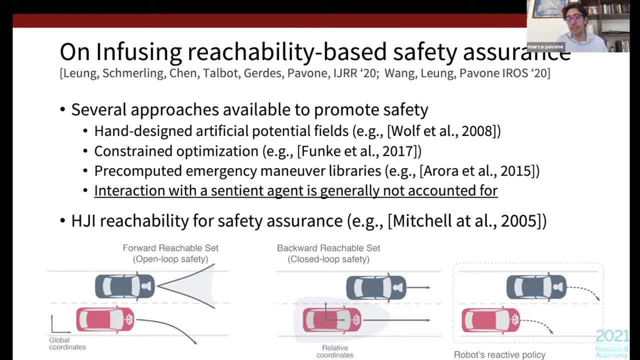 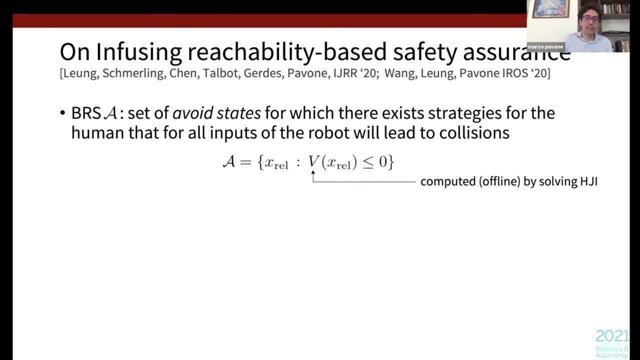 I try not to be in that situation and if I am in that situation, I try to get out of it as soon as possible. These sets where you're basically boxed in are, in a layman term, the set, that is, the backward reachable set. More formally, the backward reachable set is the set of: 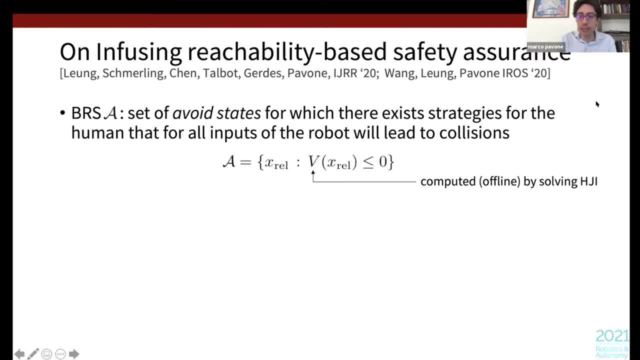 avoid states for which there exist strategies for the human that, for all inputs of the robot, will lead to collisions. In practice, this set is solved by solving a partial differential equation, referred to as the Hamilton-Yacobi-Isaacs equation, whose solution v, denoted by v the 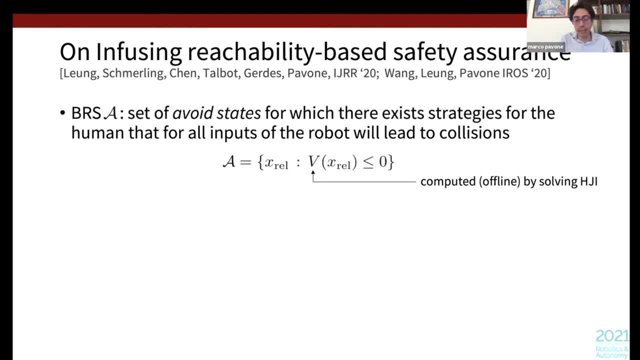 value function gives the backward reachable set as its sub-zero leveled sets. Now, computing solving the special differential equation is very complicated, but it can be done offline, fortunately. So it's not, at least from a real-time standpoint, a computational bottleneck. So the 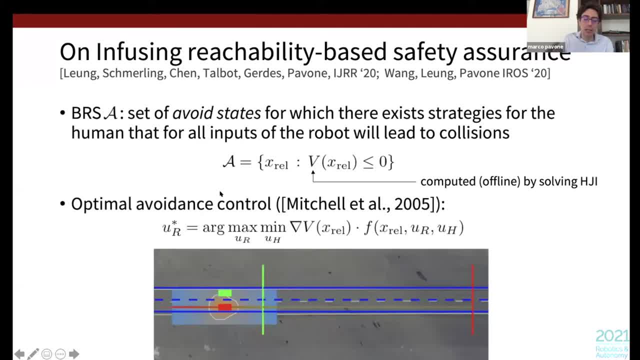 traditional application of the backward reachable set can be solved by solving a partial differential equation, but it can be done offline, fortunately. So it's not, at least from a real-time standpoint, a computational bottleneck. So the traditional application of Hamilton-Yacobi reachability to the setting of safety critical decision making. 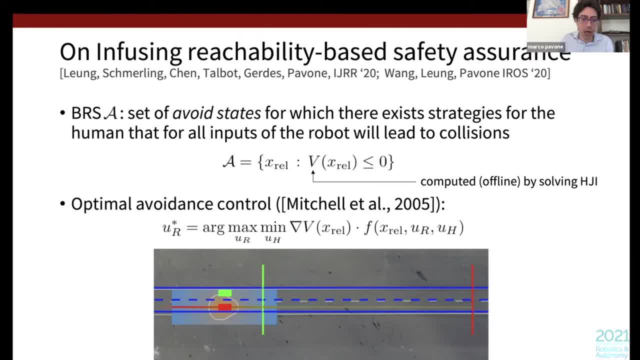 then entails computing the control u star r. subscript r stands for robot, subscript h stands for human, u stands for control. as usual in this presentation, We want to compute the control u star r that ensures the quickest possible increase in the value function, so that 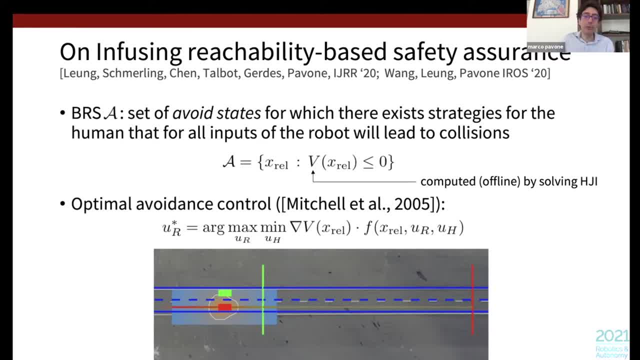 get out of the void state as quick as possible under the worst possible control or decision by a human At the bottom. I'm showing you a video about all of these works. Sorry if here the colors are not consistent, but the green vehicle represents the human-operated vehicle. the red one would be the. 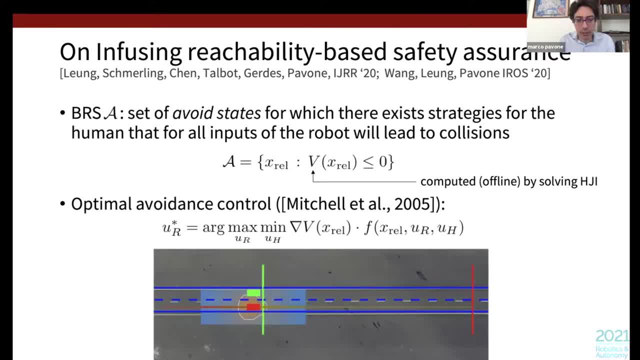 robotic vehicle. and here again we're in a case where the green vehicle is trying to swerve into the robotic one. The robotic one switches to the Hamilton-Yacobi control u star r. since now the joint dynamics are in the avoid state. 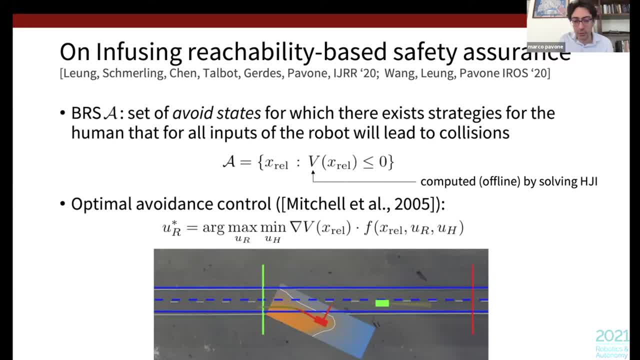 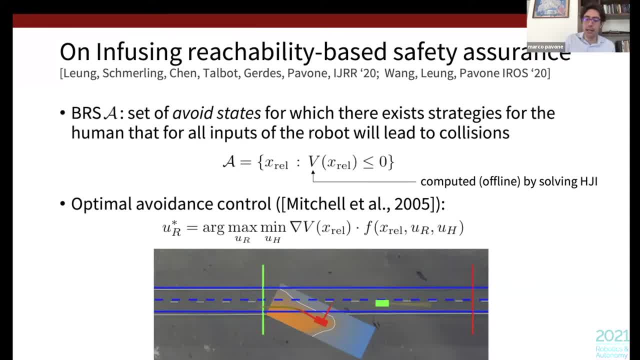 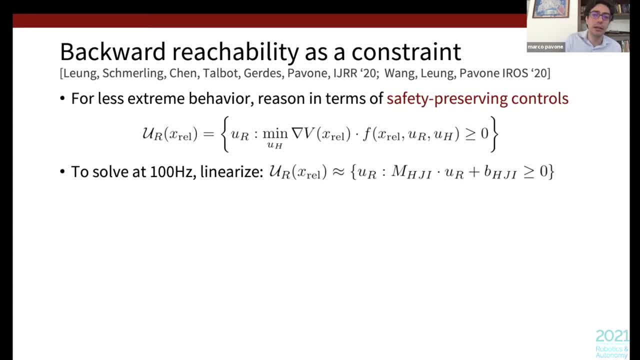 but if it is not, it will end up flying safely. From a mobility standpoint, it will be useless. nobody will get right on it. The question is: how do we retain the safety properties of Hamilton-Yacobi control while at the same time not sacrificing too much performance? well, 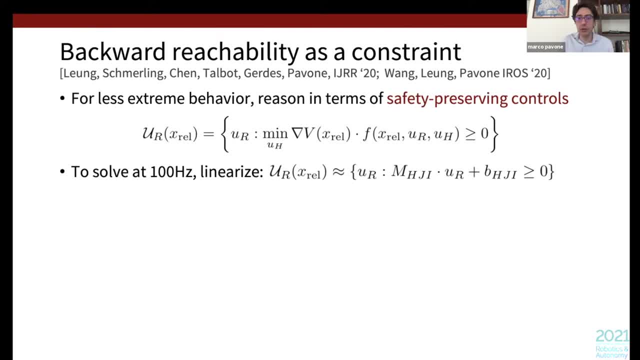 Our solution strategy is to introduce the notion of a safety preserving controls. Those are controls that ensure that the beaver at the edge of the process there is enough таol, formal integration, running out of the operation or even losing the ability to 1988 make an impact on the environment. 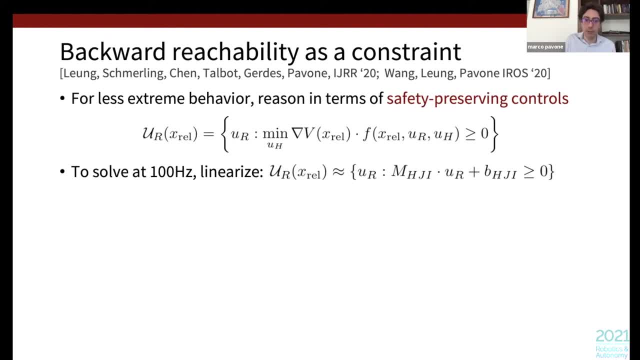 the value function is not decreasing. So with this, with controls in this set, we do not ensure that the value function is increasing at the fastest possible rate, but at the very least we make sure that the situation is not going to get worse. 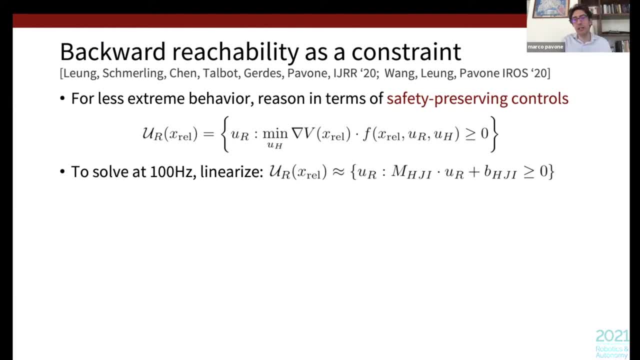 Now, this set of controls is, in general, highly non-convex, so difficult to do optimization over. So, in order to enable computation at 100 Hertz and beyond, what we do is to linearize it around an operating point and reduce the constraint of a control belonging. 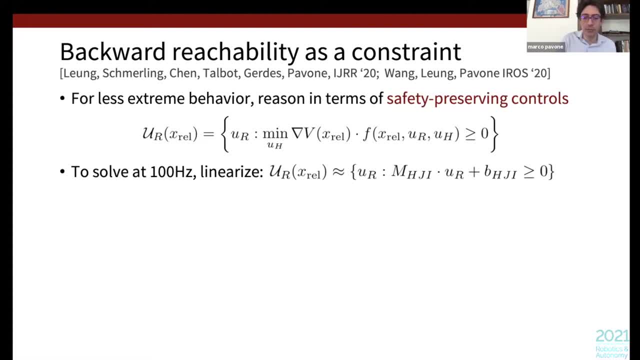 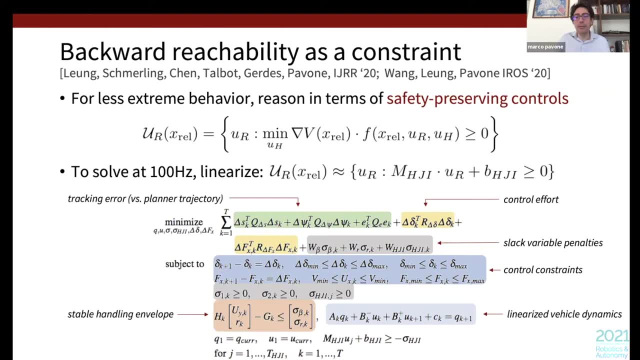 to this set and simply a linear, fine constraint, We're now in a position to present the optimization problem that brings together high level decision making and low level collision avoidance. Specifically, the idea is to set up a relatively standard model predictive control problem where the goal is to track the path that 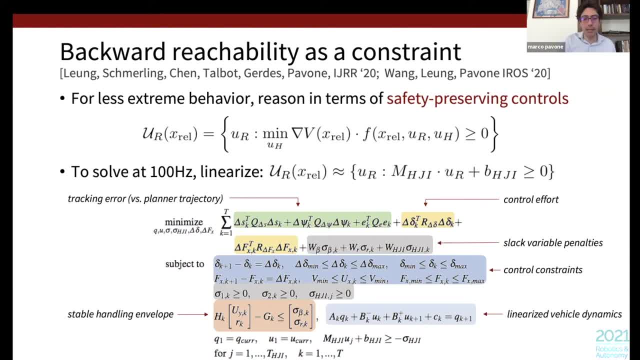 or actually the trajectory that is computed by the high level decision making model that is reasoning probabilistically in order to promote efficiency. Specifically, the cost is a traditional tracking cost, whereby we are tracking state variables like, for example, in terms of a position and heading. 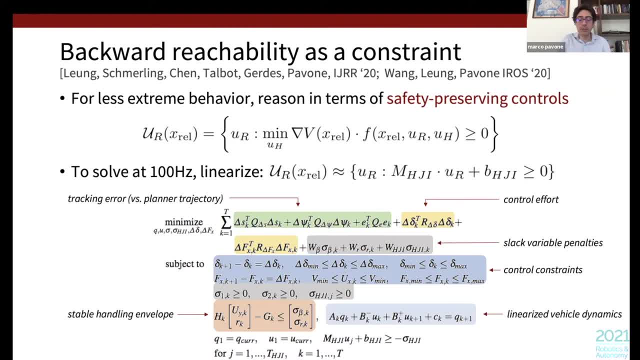 we're also taking into account, to control effort, subject to linearized dynamics, subject to linearized dynamics. subject to linearized dynamics, vehicle control constraints, stable handling envelope constraints and, critically- and this is the novelty of this work- subject to an additional constraints which forces: 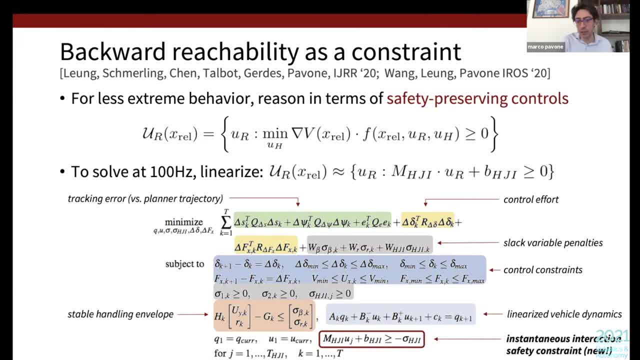 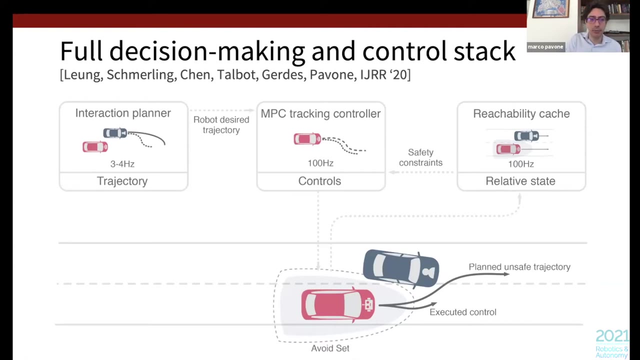 the controls to belong to the set of safety preserving controls whenever near the boundary of the backward reachable set. So, basically, these additional constraints boxed in red enforces collision avoidance in the sense of Hamito-Yokobi reachability. So, to put everything together, the full decision-making control stack that we propose entails an interaction. 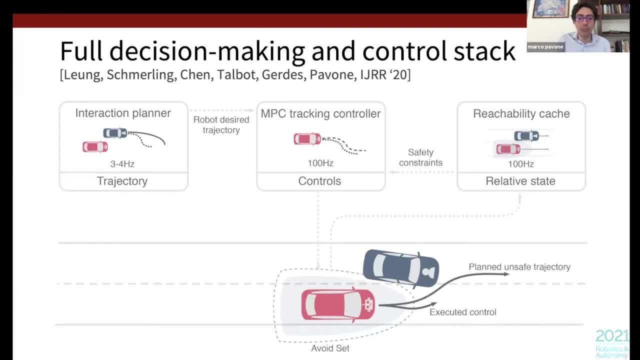 planner that produces nominal trajectories at, say, five hertz, by accounting for predictions of other agents on the road, By using a conditional variation. out-of-color model. that's a box on the left-hand side. On the right-hand side we have a reachability cache that encodes the notion of relative. 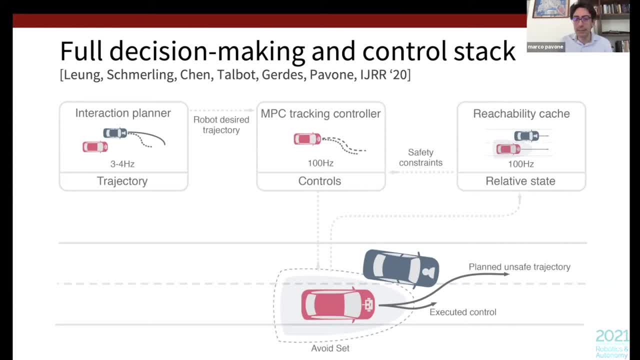 states that are dangerous in the sense that might lead to a collision despite our best effort. And finally, we have MPC tracking controller that computes controls that minimally deviate from the planner. So let's talk about the selection of the optimal policy. The conclusion is that the set of settings in a random search query can support a random 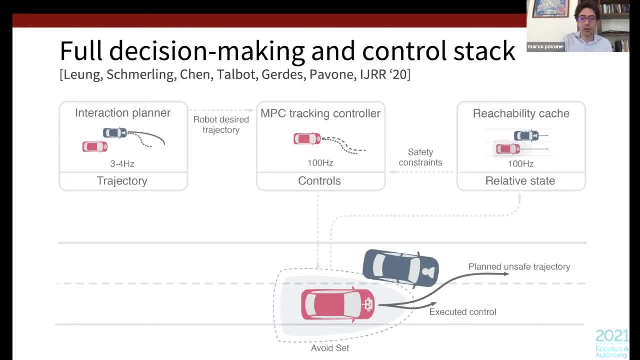 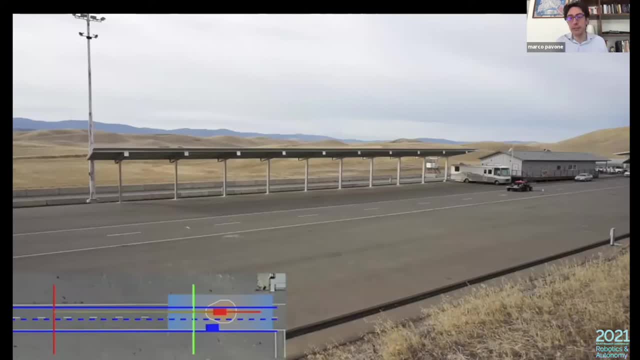 choice when ever near the backward reachable set. So let's see how all of this works. In order to test this full control and decision-making pipeline, we have used the full-scale self-driving car that we have at the lab in the Kodak center for Automotive Research Stanford. 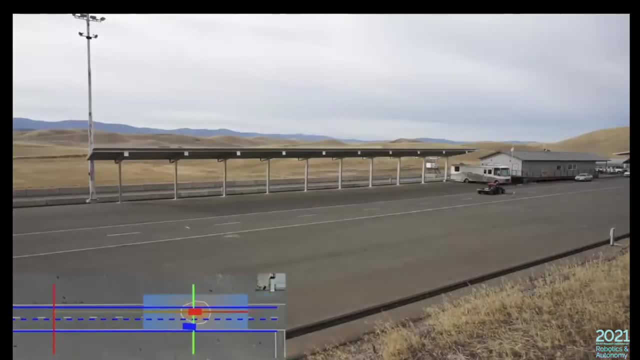 So the vehicle that you can see on the top left with the red roof is completely automated. automated so the perception and the interpretation, decision-making, low-level control. These are basically the algorithms that I presented today. The role of the human vehicle is taken by an RC. 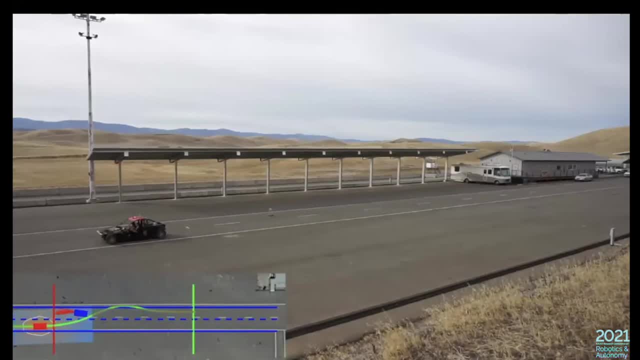 car, the small car with the white mast that you see. The reason why we have this white mast on top of the RC car is to make sure that it's visible from the ladders on the self-driving car And that the RC car is remotely controlled by a student. The reason why we use an RC car is that 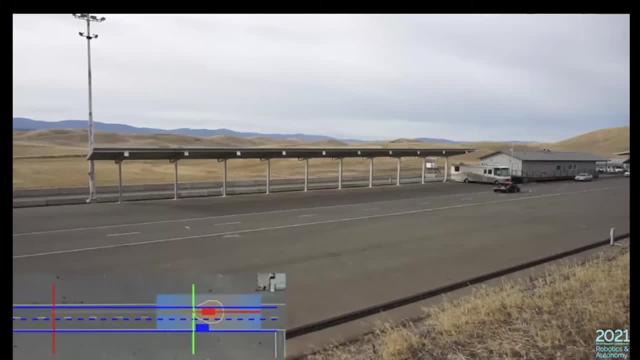 basically, we're asking the student to abuse of the algorithms, to behave in a way that is completely erratic, and so, for safety purposes, we don't want to use a car with a human on it. So here again, it's an example whereby the goal is again traffic weaving: swap lane On the bottom left. I'm showing. 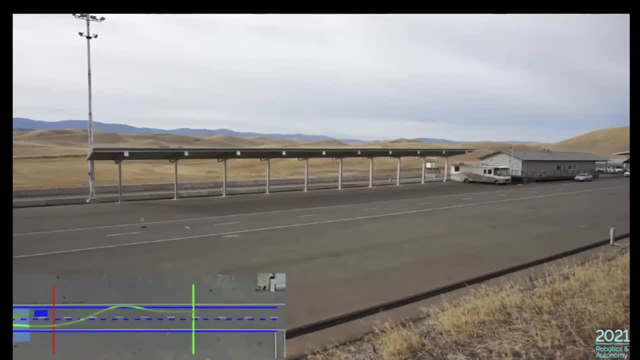 the video interaction with a top-down view. The red vehicle here is the robotic one. the blue vehicle will be the RC car. So this is the setting whereby initially the human, so the RC car, is driving nominally, so it's going straight and all of the sudden it decides to swerve into us, As you can see. 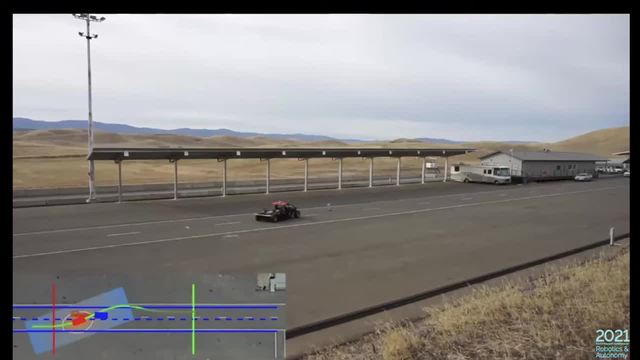 here the self-driving car reacts quite smoothly by just gently getting a little bit outside the road, accelerating and completing the motion. So relatively fast interaction. so here the vehicles were going at about 20 miles per hour, 25,, very uneventful, and it's the point of this video to show how such a relatively complex interaction. 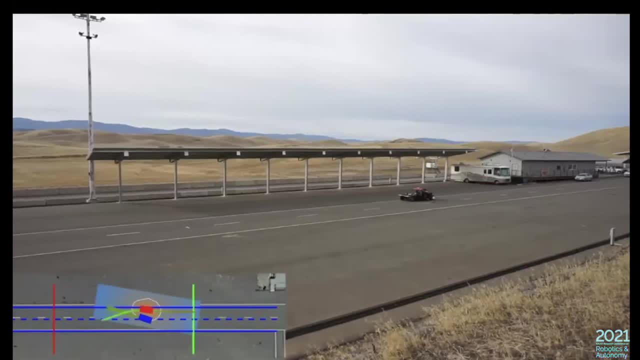 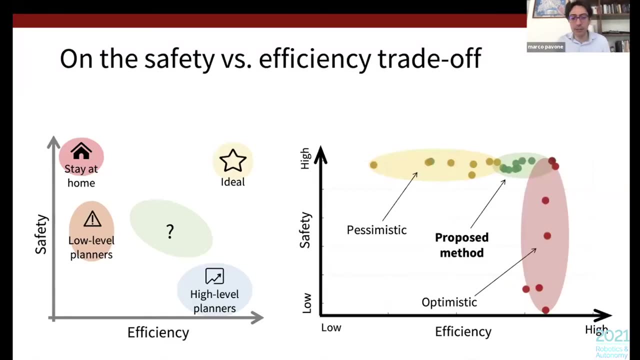 plays out very naturally smoothly with the right balance, at least qualitatively in terms of safety and efficiency. But it's a little bit more quantitative about this balance between safety and efficiency On the left-hand side. here I'm showing you the conceptual plot that. 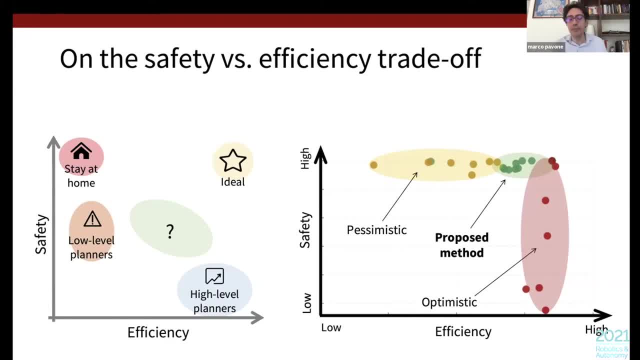 I showed you before. On the right-hand side, I'm showing you the actual results from the field tests. Now we could talk at length in terms of what are the best ways to measure safety or efficiency In our work. we measure efficiency by taking into account. 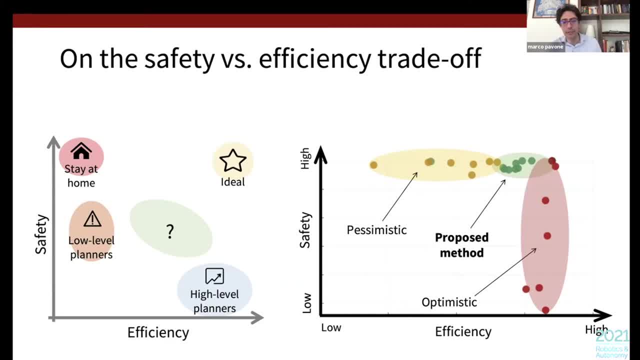 g-forces, which are basically a proxy for comfort and the control effort and for safety. we measure safety by accounting for how close we came to penetrating the backward reachable set. So we benchmark our proposed method against a pessimistic and against an optimistic controller. 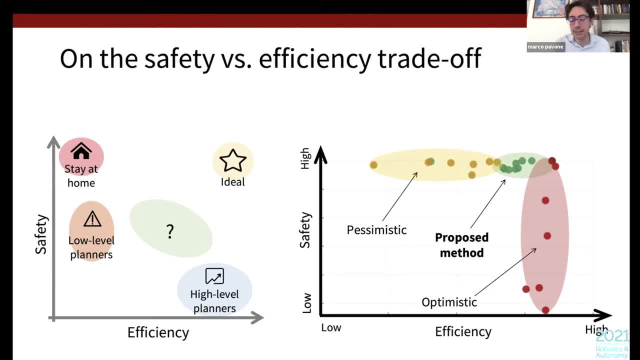 The optimistic controller is the one that runs the trajectories as computed by the high-level decision-making models without accounting for low-level collision avoidance. The pessimistic algorithm is the one that has a low-level collision avoidance. algorithm that entails switching abruptly to the Hamilton-Yakovsky. 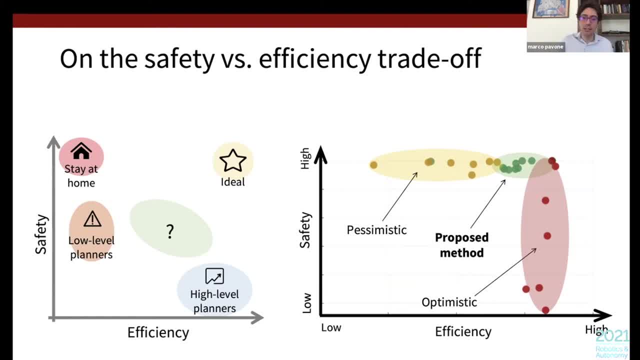 control. So, as you can see, the pessimistic controller is typically extremely safe, but sometimes not very efficient. Not efficient basically means that the vehicle stopped at the side of the road. The red represents the performance of the optimistic algorithm and here you can see that typically very efficient. so when it completes the maneuver, it 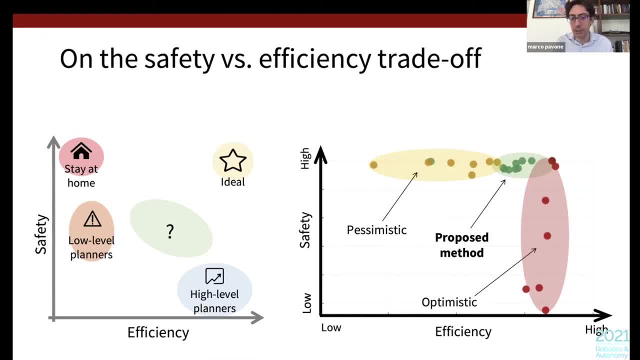 completes it very quickly, but sometimes it leads to collision, And the green dots represent the result of our method. and here, basically, we achieved our goal of achieving the goal of the goal of really blending the efficiency and safety of the two different competing priorities. 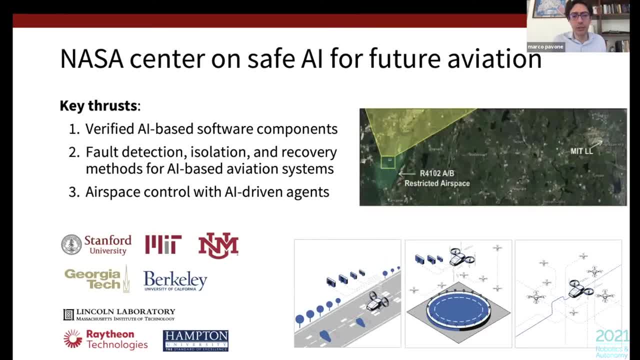 So this was very satisfactory for us and it's actually related to a new project in my lab, which is a fairly large project funded by NASA in collaboration that I'm leading in collaboration with a number of other universities such as MIT, Georgia Tech. 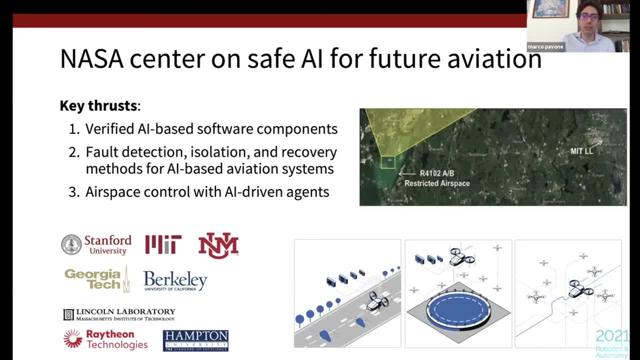 Berkeley and so on and so forth, which is focused on safe AI for a future aviation system. So we're going to take this work to the next step in terms of complexity and also apply it to aviation systems. Specifically, we are focused on three research trusts. The first one is 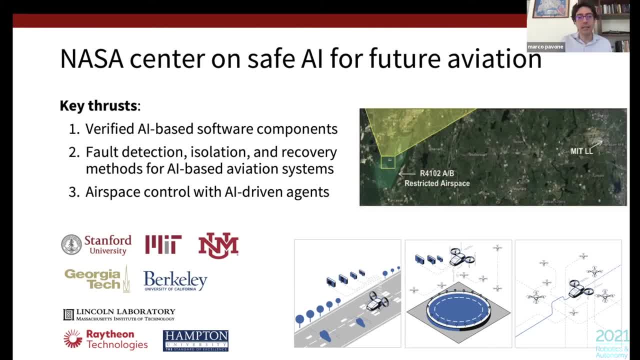 offline assurances. so how to build data-driven methods for autonomy stacks that come with some guarantees? The second trust entails online assurances. How do we monitor those components of the autonomy stack that rely on data-driven components In such a way that we can trigger anomaly signals in case a given component is misbehaving? 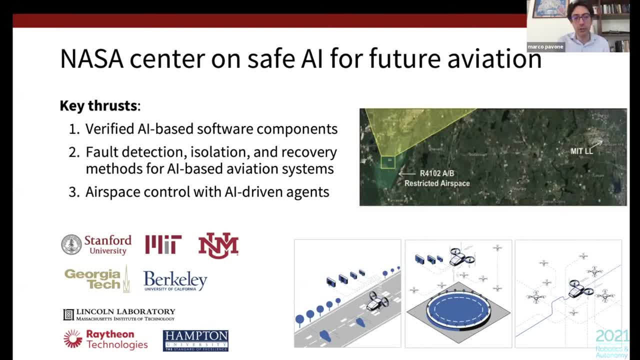 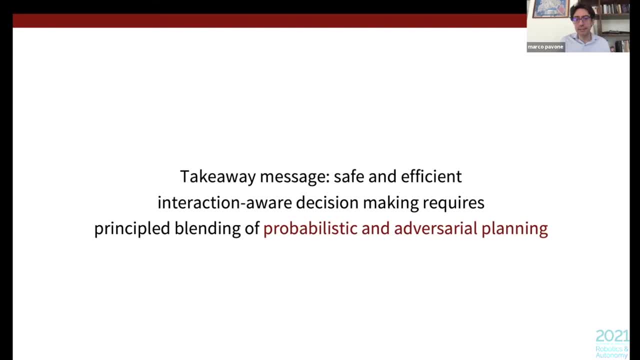 And, finally, how we reason about aerospace control when some of these agents are AI-driven. The takeaway message of this second part of the talk is that safety-efficiency interaction over decision-making requires principle blending of probabilistic and unrecycled planning. We're now working on a number of ways to extend this work, particularly 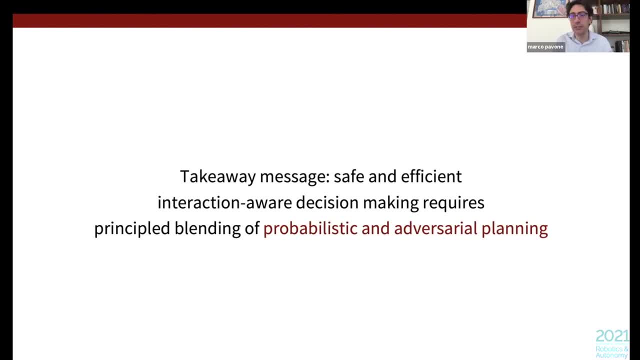 how to come up with representation for forecasting trajectories that are more conducive to downstream decision-making. Two, how can we account for uncertainty that stems from upstream perception models. And three, how we embed logic, or, if you will, symbolic reasoning, in data-driven models in order to embed some notion of interpretability and causality. Fortunately, I 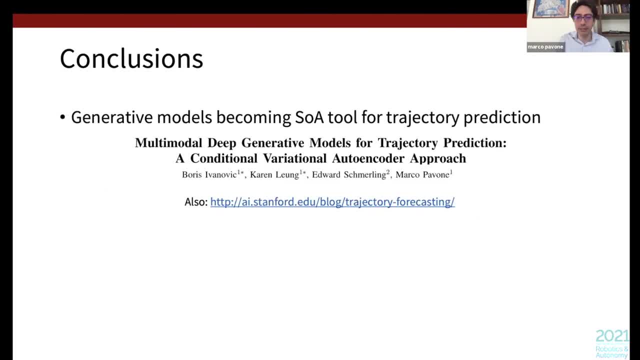 will have to skip through these three topics. If you're interested, I'd be happy to cover them in the Q&A session. Let me conclude by saying that the journey models are becoming a state of the art tool for trajectory prediction. If you are interested in this topic, we have